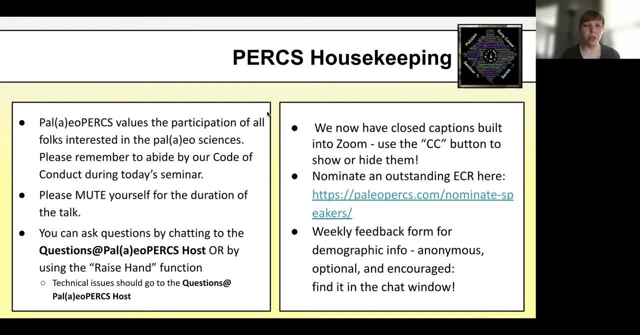 So some quick housekeeping things. Paleo Perks values the participation of everyone interested in the paleo sciences, so please remember to abide by our code of conduct during today's seminar. You agreed to it when you signed up. If you found yourself here without having signed up, 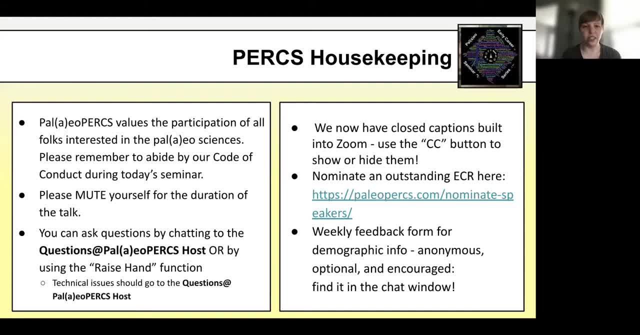 For the mailing list. You can check out the mailing list or sign up for the mailing list on our website and quickly look over the code of conduct as well. So please also keep yourself muted for the duration of the talk And following the talk. as we said, you can ask questions by chatting to the questions at Paleo Perks host or, if you'd rather, by using the raise hand function and we'll unmute you. 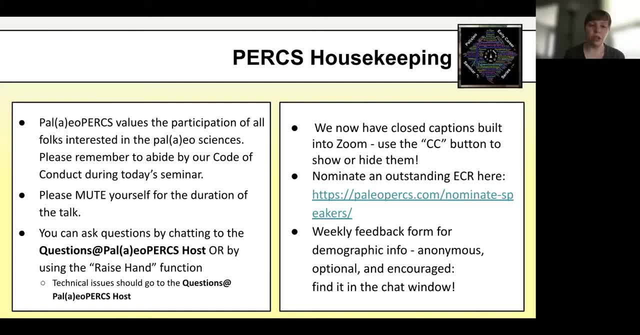 Then if you want to ask your questions Out loud. Additionally, if you have any technical issues during the talk, you can send those via the chat to the questions at Paleo Perks host as well. So we now have built into zoom. you should be able to use the CC button to show or hide them. 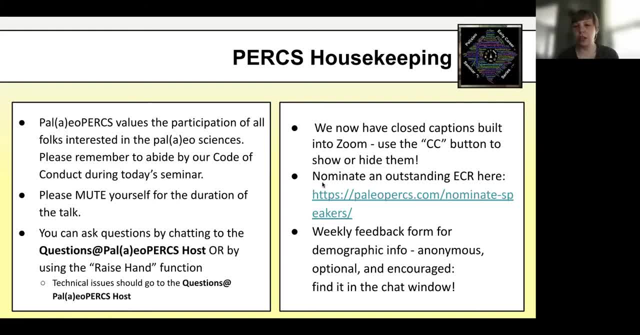 Additionally, we're always looking for nominations for other early career speakers and we'll drop the link for where you can nominate someone in the chat. Also into the chat will drop our weekly feedback form that just collects demographic information so we can get an idea of who's attending. it's anonymous, optional and encouraged. 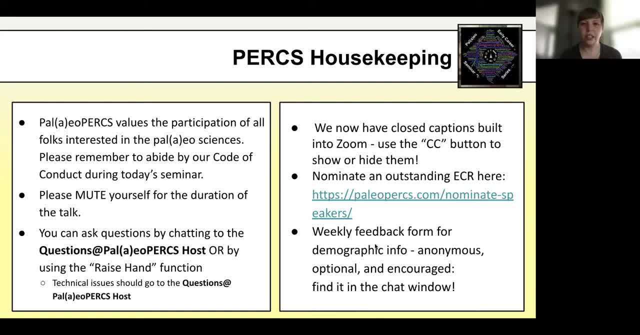 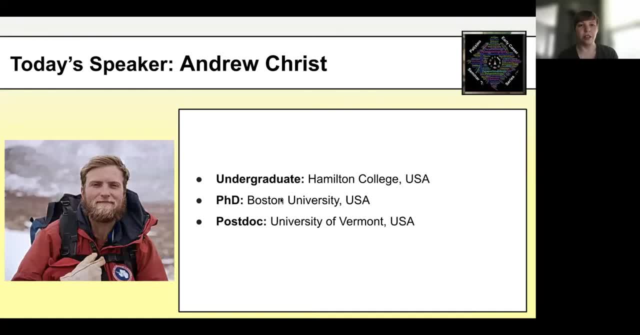 So please fill that out really quickly As you see it pop up in the chat. So today's speaker, as we mentioned, is Drew Christ, who is currently a postdoc at the University of Vermont, After having gotten got his undergraduate at Hamilton College and a PhD at Boston University. and Drew is going to 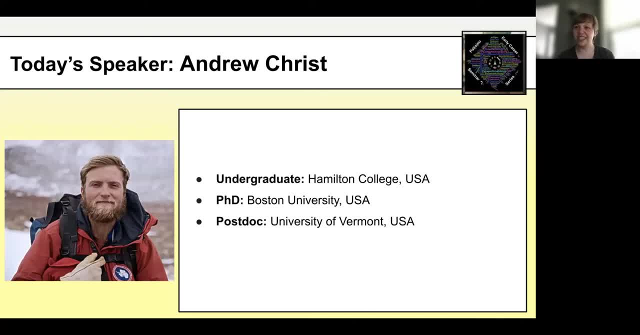 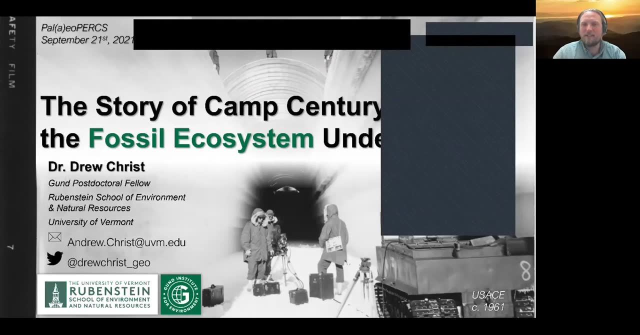 talk to us about some ecosystems under ice. so if you want to take over the screen, share, Drew. I'm really excited to see what you've got for us- Awesome. thank you so much, and thanks to the organizers for putting on such a great series. it's really wonderful to see all. 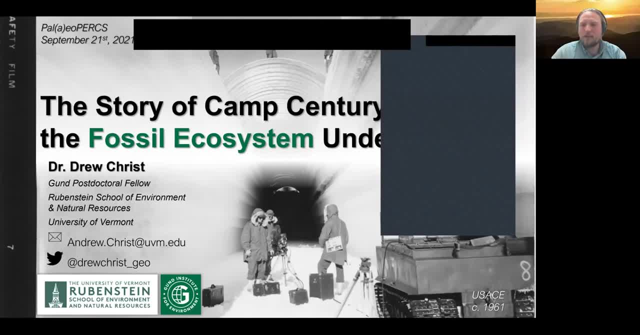 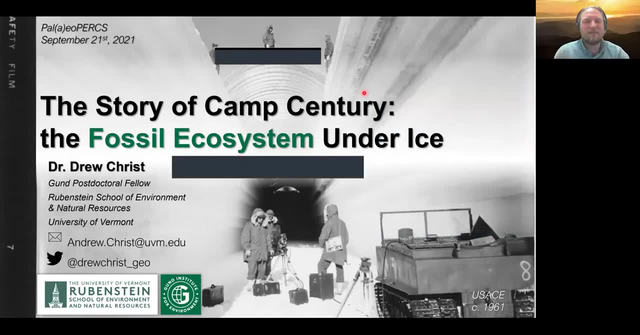 these people from around the world sharing their research and getting to be amongst other early career researchers is really great, because it feels like a good space where we can all share our ideas and support each other. so thank you guys, so much for organizing So today I'm 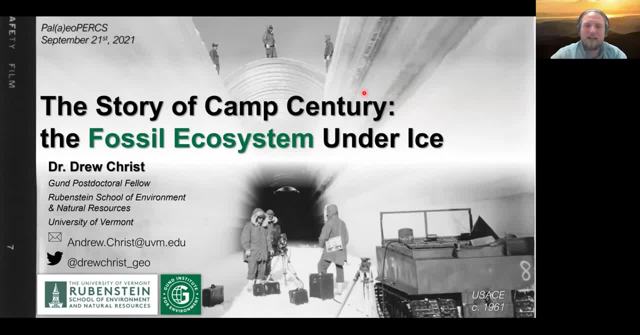 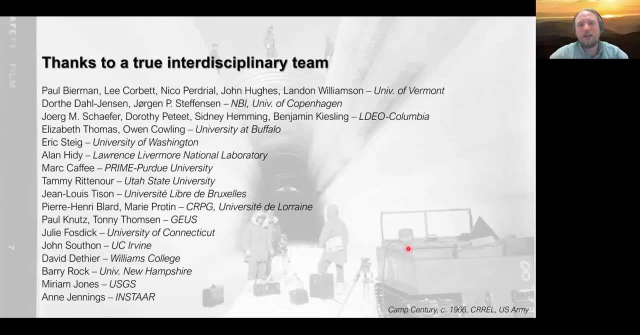 going to be talking about the Camp Century Ice Core, specifically the sediment from the very bottom of it and the fossil ecosystem that we found in that sediment. So, before I get too far along, I just want to acknowledge that this is a project that has been made possible by many, many different people, who. 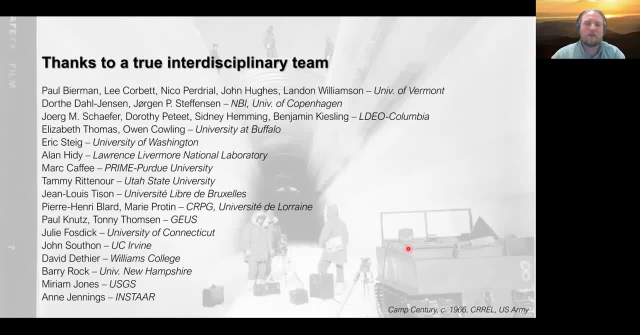 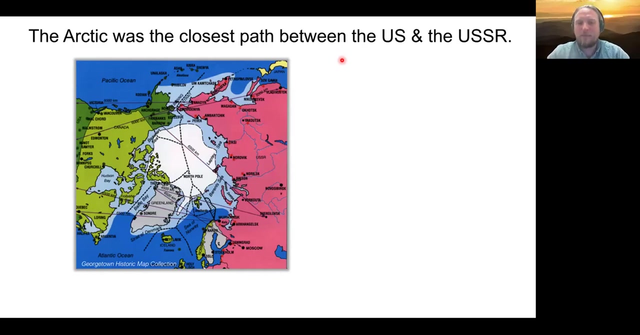 are either contributing samples or analyses or just expertise in ice core science, and so this is really a huge team effort and I'm just very privileged and lucky to get to work with these people and learn from them. So you can't talk about Camp Century without talking about history, because the whole reason 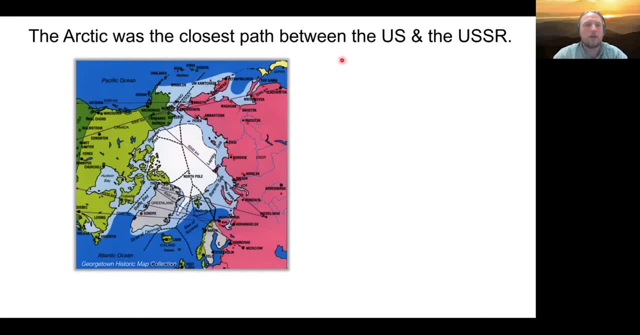 that Camp Century exists is because of the Cold War, and so at the height of the atomic age during the Cold War, the Arctic was the closest path between the Soviet Union and the United States and the Soviet Union, And so there was a huge worry that there were going to 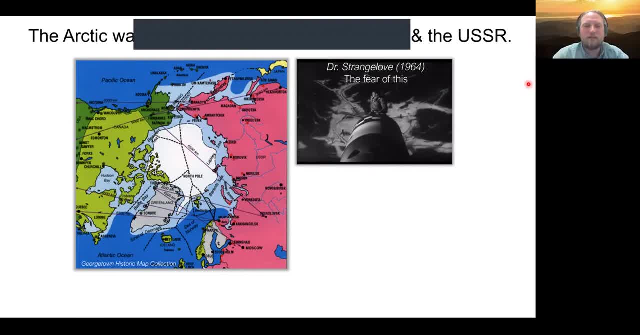 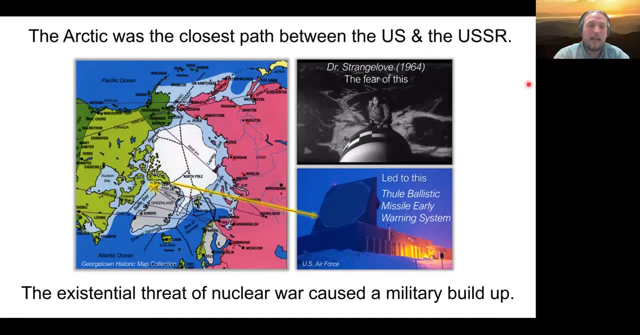 be intercontinental missile strikes shot across the Arctic Ocean from the Soviet Union to the United States. This led up to a military buildup among the NATO nations in the Arctic, and the US Military, with permission from Denmark, built a large air force base in Tule, and the US military, with permission from Denmark, built a large air force base in Tuly, but with only this level of ai. 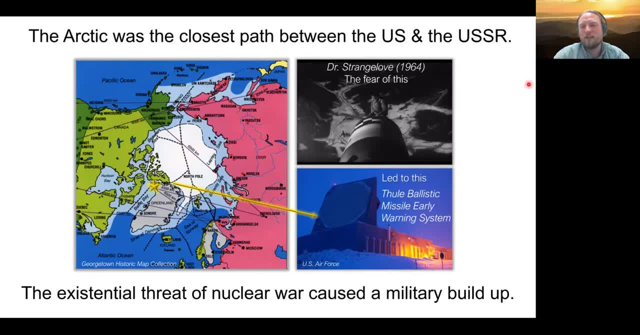 gs' bullshit. So this was a mistake I made about how the Irish people were able to get to Earth from here. But by the end of the 1985 Somerset movement there was a very serious in northwestern Greenland where they installed this early detection missile warning system that 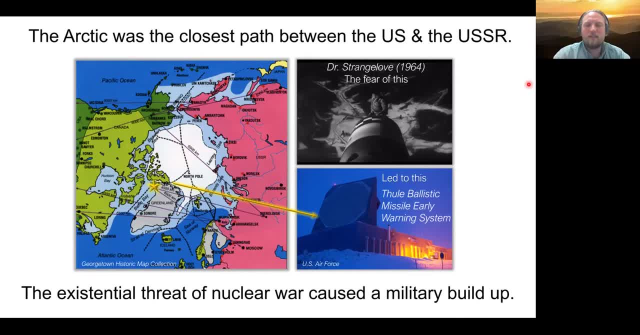 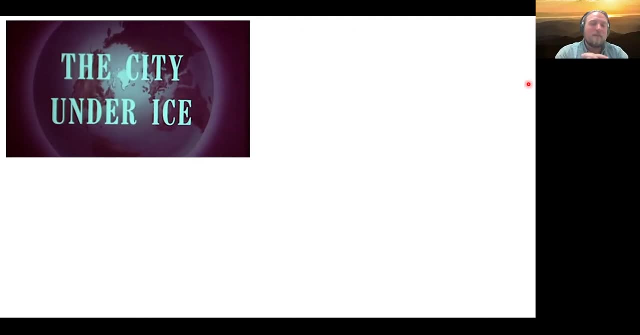 is still there today. And so, as the US military was building up military operations in the far north, they started to do some kind of wacky things, And among the craziest things that the US Army did during that time was build Camp Century, which was this city under the ice. 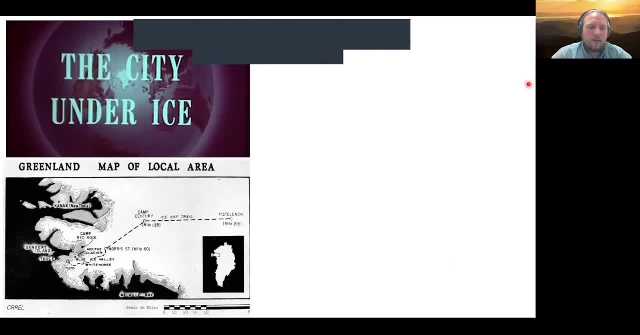 So in the late 50s the Army started hauling heavy equipment with snow cats across the Greenland ice sheet about 100 miles into the interior from Thule and started digging a series of tunnels into the actual ice and snow to build a military base. 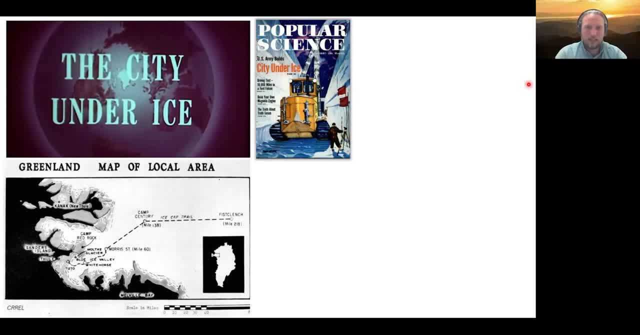 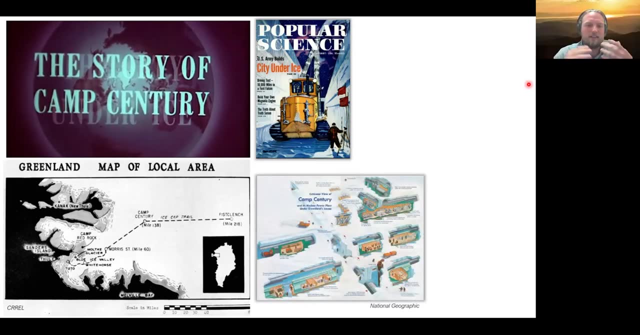 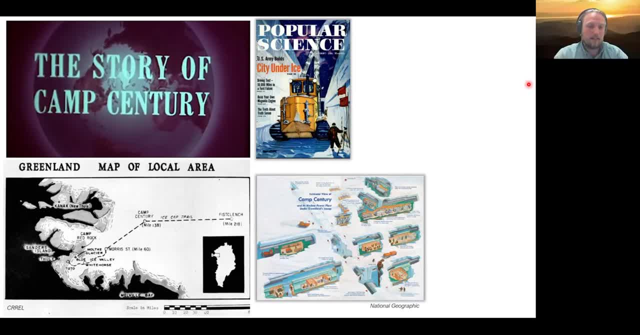 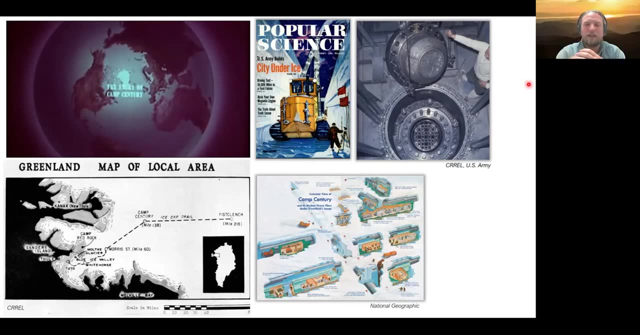 highly public to the Americans and other western nations through popular media like National Geographic, Popular Science. They even brought up Walter Cronkite, the CBS news anchor, to do a 30-minute long news film about Camp Century. And because this was the atomic age, they also decided to power this base with a small nuclear 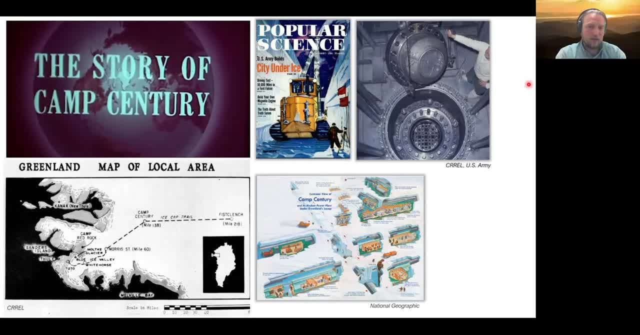 reactor And that could support up to about 100 soldiers, engineers and scientists. Now, the real reason behind why the US Army was interested in building this base was that there was this project, or secret mission, rather called Project Ice Worm, where the military was. 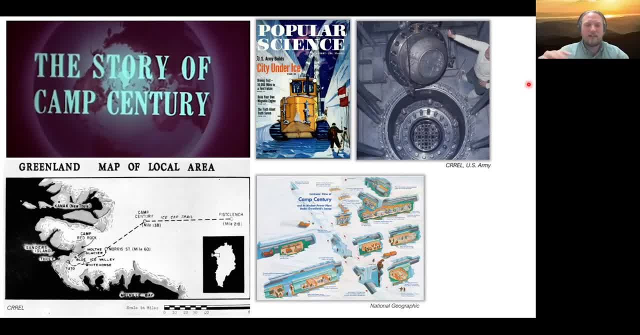 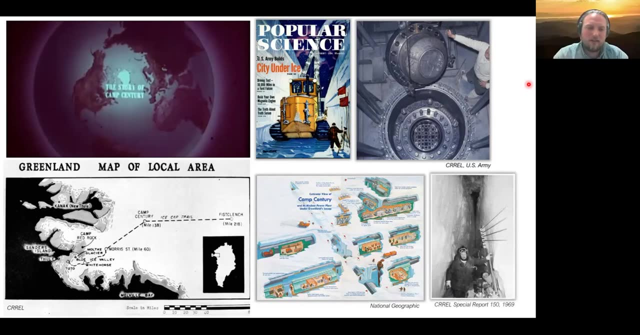 devising a way to build a series of railway tunnels inside the ice sheet so that they could store and hide nuclear weapons from the Soviets. So the Army very quickly learned that that was not possible because, as we know, ice sheets are these flowing masses of ice that deform over time. 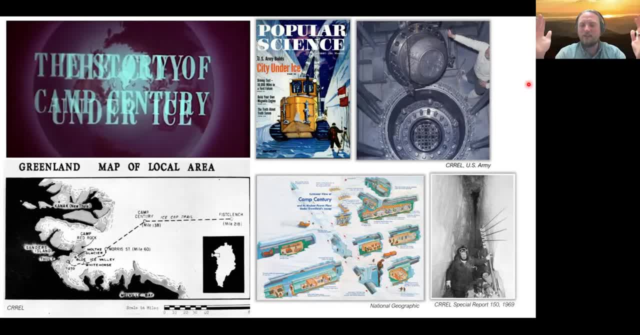 And so, as they were occupying the base, they were able to build a series of ice sheets that were They started to realize that the walls were starting to collapse in, either from the ductal deformation of the ice itself, as well as the really high snowfall rates from above that we're starting to crush buildings. 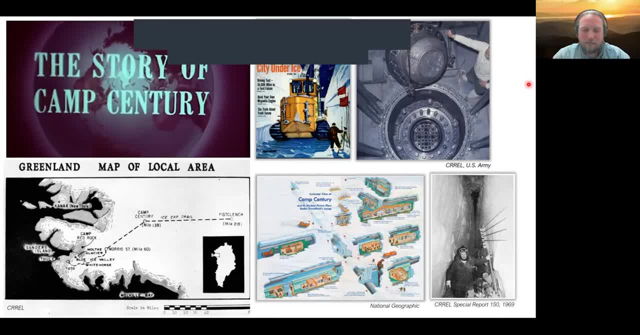 So after 1966 they abandoned the base and only a few years later they went back and saw that this tunnel that would be wide was now only about four feet wide because everything started to compress. So while this was this kind of crazy Cold War science fiction-esque project, they were actually doing some incredible basic science at Camp Century. 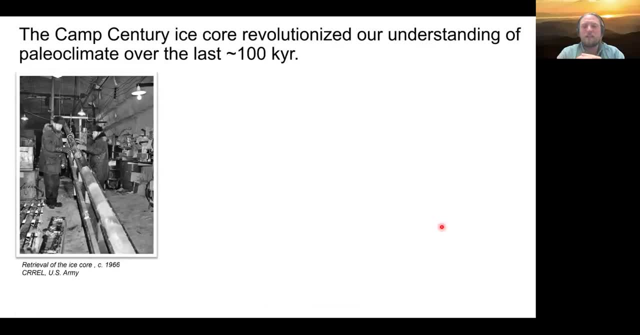 And one of those projects was studying the ice sheet itself And they collected the very first ice core drilled through the entire thickness of an ice sheet at Camp Century And the analysis of that ice core really revolutionized how we understand Earth's climate over the last hundred thousand years. 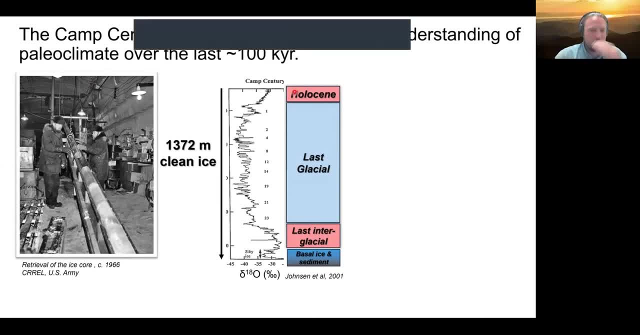 Within the ice core we were able to see the entirety of the Holocene, the last glaciation, the last glacial and all the interstadials and rapid climate changes during the last glacial period back into the last interglacial. 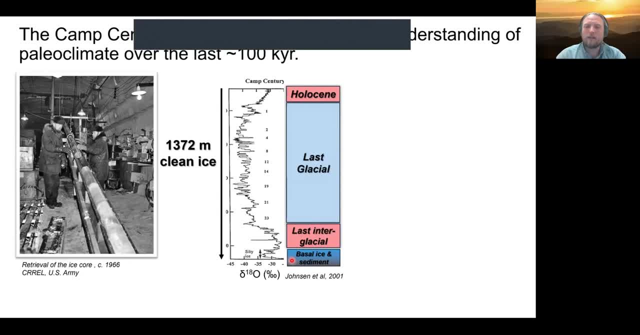 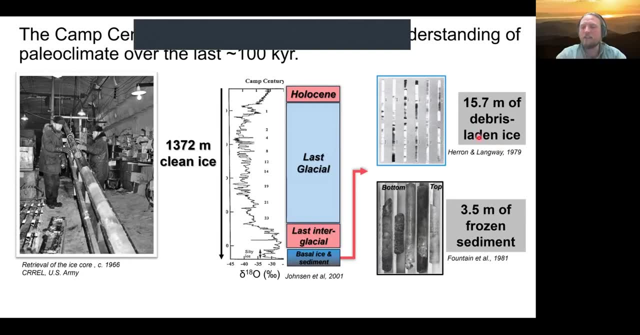 And then, at the very bottom of the ice core, they recovered basal ice and sediment, So about 16 meters of debris-laden or sediment-laden ice. So about 16 meters of debris-laden or sediment-laden ice And at the very bottom about three and a half meters of frozen sediment. 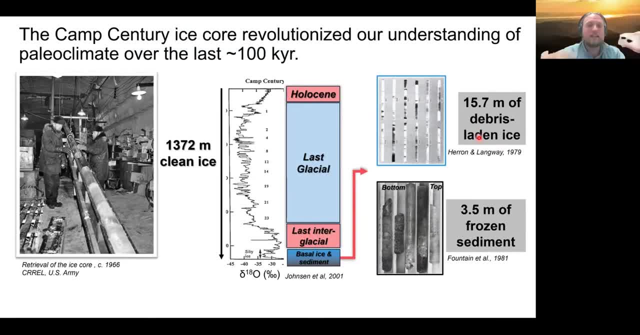 So the ice core, the actual ice, was studied intensively and extensively, But these basal materials were not studied very much And then they were actually lost for decades. So they were initially in the US at the University of Buffalo until the late 80s, early 90s. 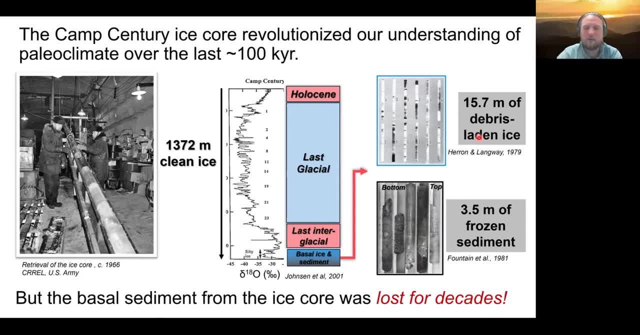 And then they were shipped over to Denmark to the Niels Bohr Institute, And then they were shipped over to Denmark to the Niels Bohr Institute, Where they kind of just sat in a cold dark freezer for the last 30 years until they were rediscovered during an ice core inventory. 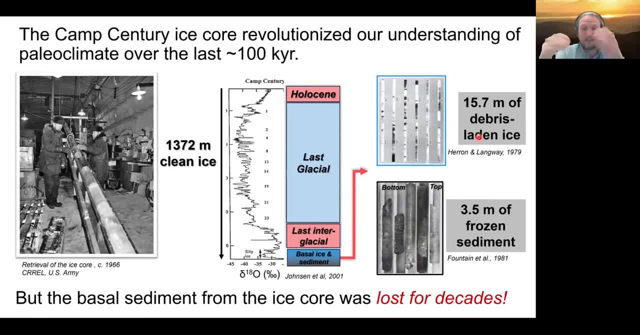 Where they kind of just sat in a cold dark freezer for the last 30 years until they were rediscovered during an ice core inventory. And so the group of scientists I'm working with, we were all kind of tapped to come in and supply analyses for these. 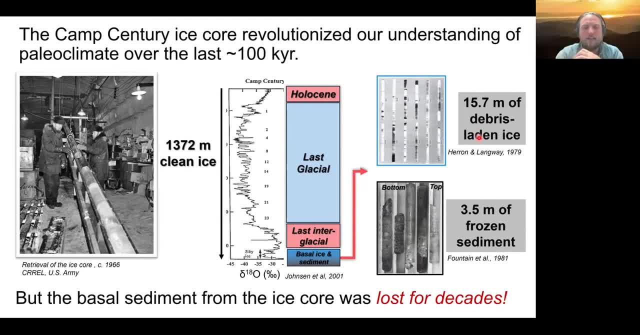 And so the group of scientists I'm working with, we were all kind of tapped to come in and supply analyses for these, And my advisor here at UVM, Paul Bierman, who specializes in cosmogenic nuclides, thought that this would be a great project to do. 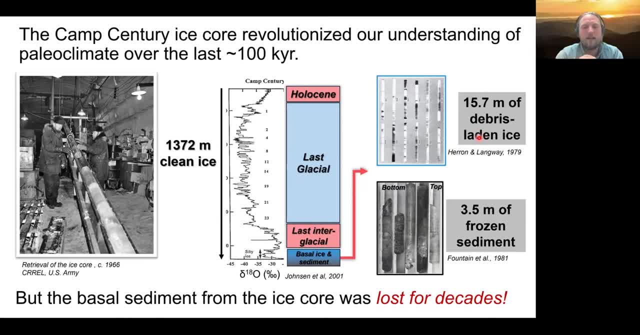 And my advisor here at UVM, Paul Bierman, who specializes in cosmogenic nuclides, thought that this would be a great project to do at UVM Paul Bierman, who specializes in cosmogenic nuclides, thought that this would be a great. 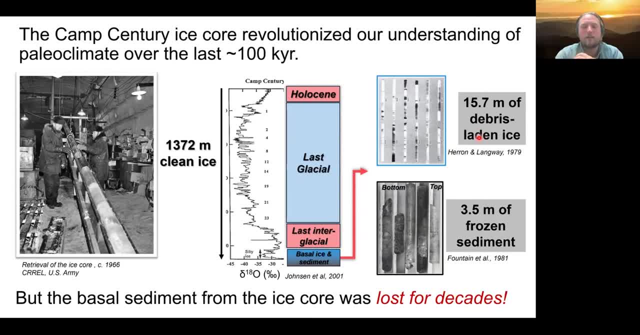 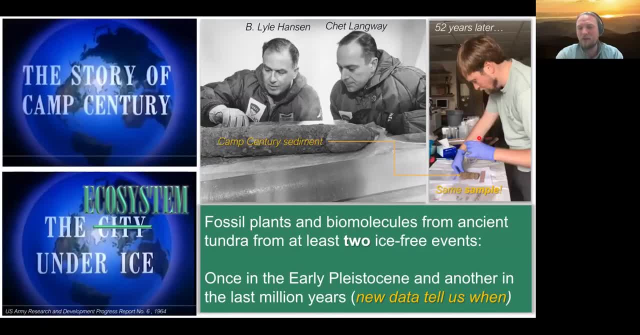 project for me to work on during my postdoc, And it turned out to be a really incredible project, because we didn't really know just how cool this was going to be. So the story of Camp Century isn't just a story about the city under ice. it's really the ecosystem under ice And separated by 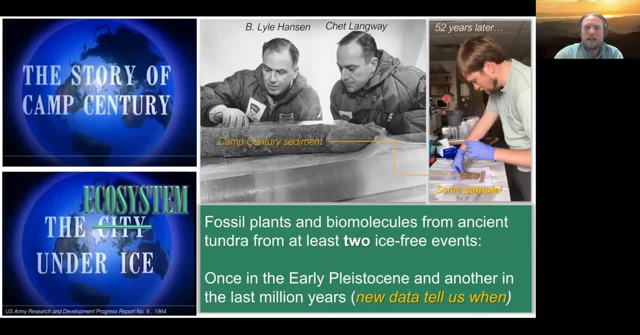 almost 60 years. we are able to go and look at the basal sediment from Camp Century shown here, with the original ice core scientists Lyle Hansen and Chet Langley back at this Pentagon little photo op in the late 60s to me working on the exact same sample of sediment over 50 years. 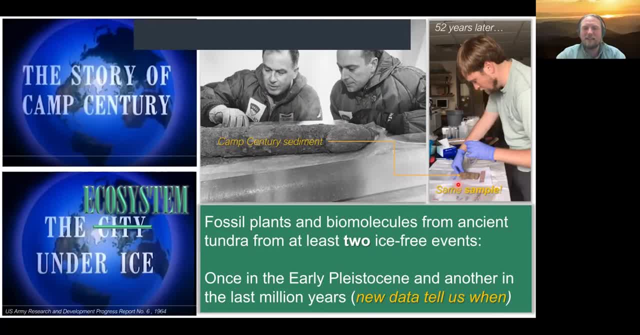 later, And what we just is that it contains fossil plants and biomolecules from ancient tundra, from at least two ice-free events in the past, Once in the early Pleistocene and another in the last million years- And we have some new data that tells us when that last event 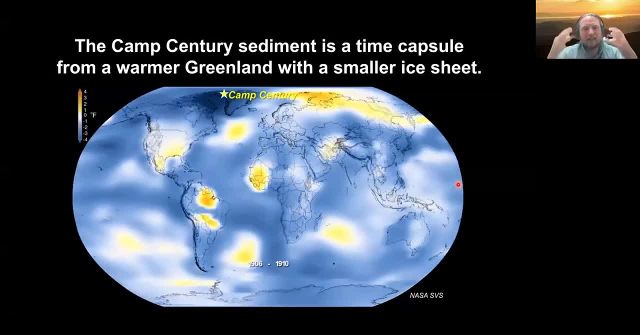 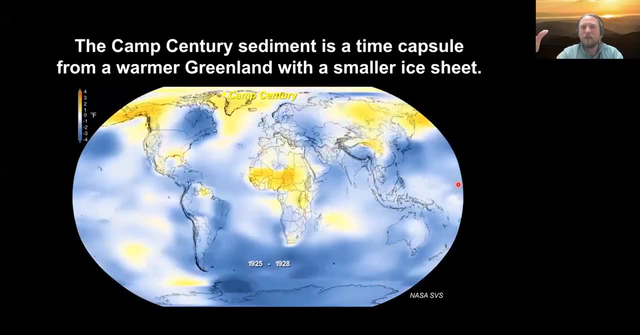 may have been. So this Camp Century sediment is really a time capsule, because it tells us a tale of a warmer Greenland, when the ice sheet was smaller than it is right now, And this, of course, is important as we look to the future, as humans continue to warm the climate. 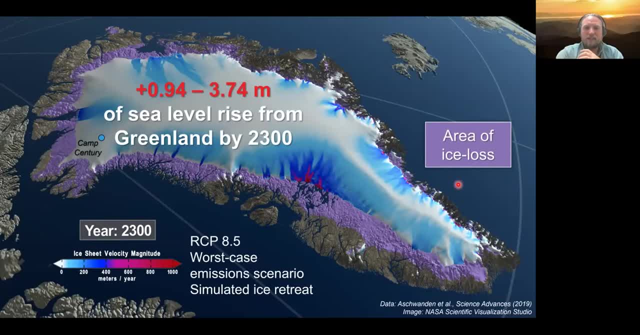 and melt the Greenland ice sheet In the next couple of centuries. if we continue on our business as usual, burn all of the fossil fuels in the ground approach. we could melt significant portions of the Greenland ice sheet and raise sea level as much as 3.74. 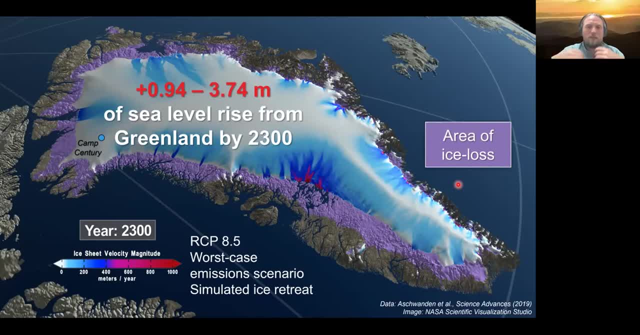 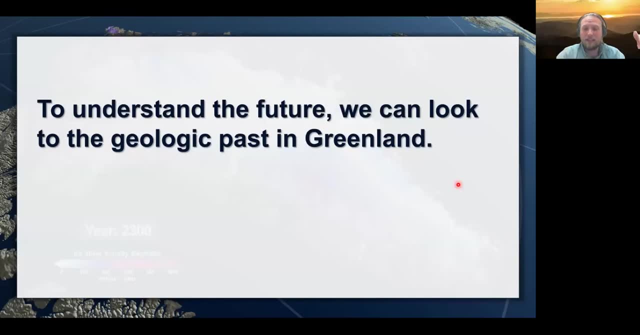 meters. So we want to understand the future right. What is the fate of the Greenland ice sheet? So we can look to the geologic past And specifically we want to know when did parts of the Greenland ice sheet have, about 70,000 years of life, if that's at point reached, And what fast we can solve by fish, or they could dirt To. 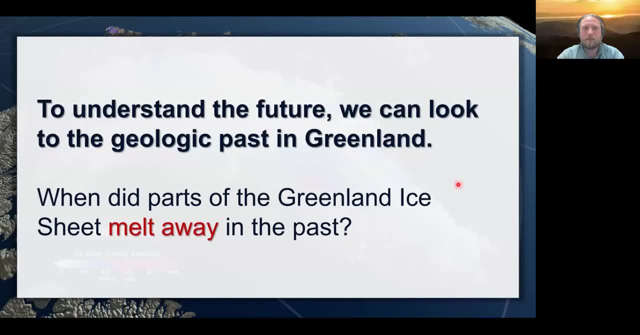 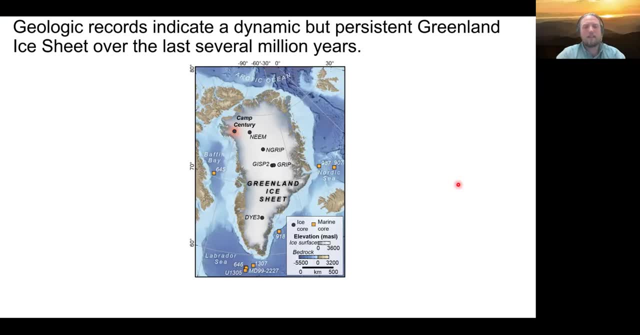 and ice sheet melt away From the geologic record. we're beginning to see that the Greenland ice sheet has been dynamic but persistent on Greenland for the last several million years. It's more or less been there, but there have been times when it has retracted in size. So we can look at the 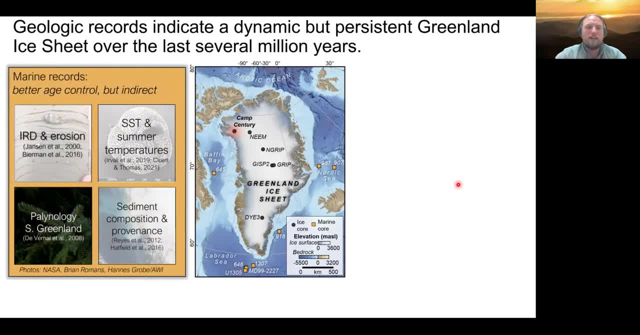 marine record, which are continuous records with oftentimes better age control. but these are indirect measures of what the actual extent of the ice sheet is right, They're proxies, So ice rafted debris can tell you about how much ice you know if there's ice terminating into. 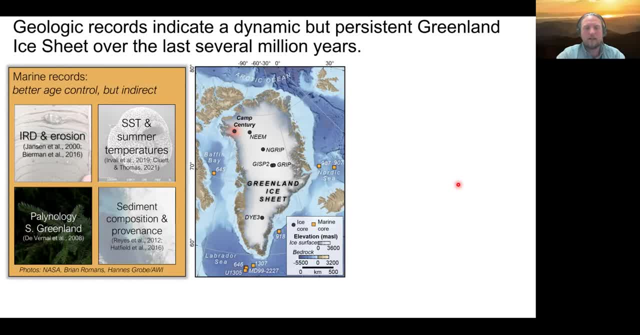 the ocean and the volume of ice rafted debris being delivered out into the marine realm, as well as sea surface temperature and summer temperature, reconstructions From micropaleontology and leaf waxes, as well as looking at the palynology and sediment. 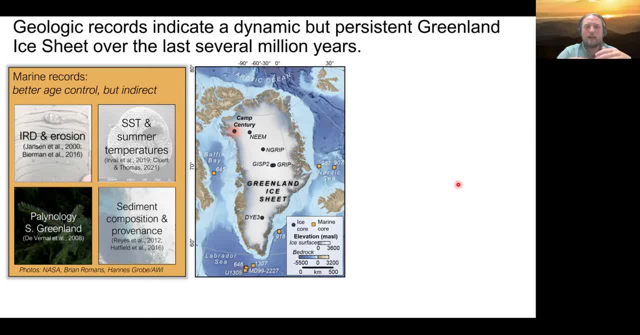 composition off of southern Greenland, which gives us an idea of whether or not southern Greenland was ice covered or not. Now the other way that we can look into the deep time record of the Greenland ice sheet is to look at ice core basal materials. These can directly tell you whether or not those 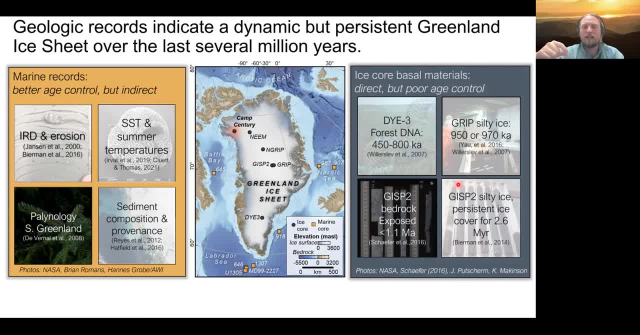 locations were covered by ice in the past, but it's been really challenging to get good geochronology on the Greenland ice sheet. It's been really challenging to get good geochronology on the Greenland ice sheet. It's been really challenging to get good geochronology on the Greenland ice sheet. 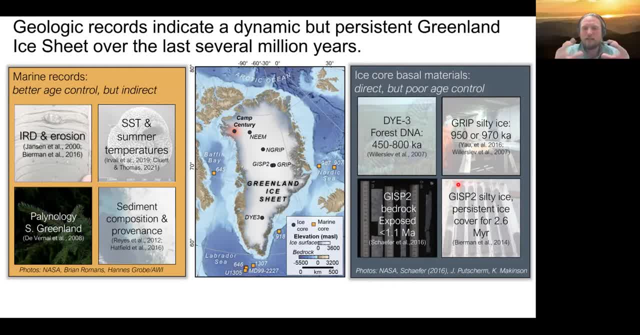 But what we have right now is an emerging picture that the Greenland ice sheet must have been absent within the last million years. And we know this because at the center of the Greenland ice sheet, at Gisp 2, the subglacial bedrock must have been exposed within the last 1.1 million years. 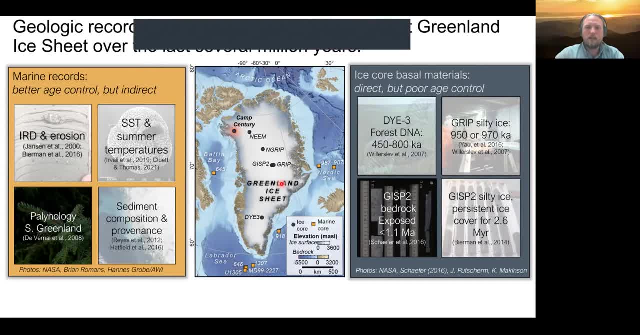 and that's using cosgenic nuclide data. We also have some evidence from the Dai-3 ice core in southern the Greenland ice sheet that shows that the ice sheet retreats from the Greenland ice sheet retreats to be boreal forests there And there's an ancient DNA analysis of that basal ice that contains flora. 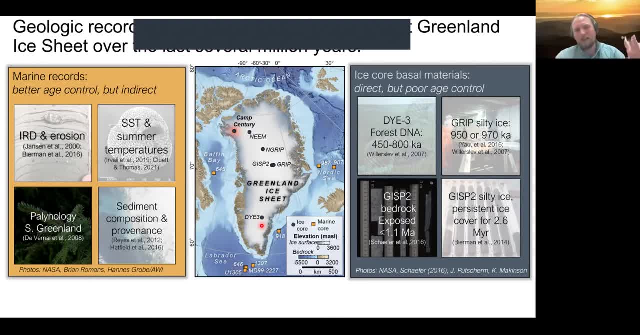 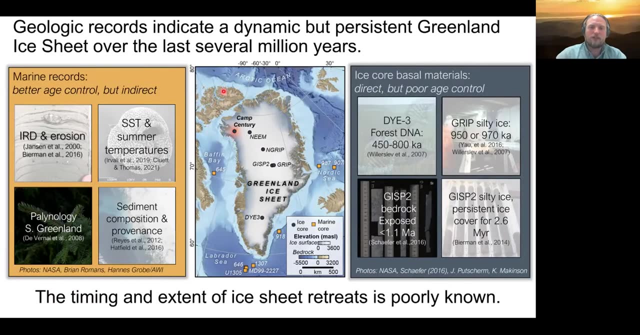 and fauna from boreal forests. So it's beginning to look like the Greenland ice sheet must have been smaller at some point in the last million years, but the timing and the extent of those ice sheet retreats is poorly known. We can go to Camp Century up here in the far northwest portion of the ice sheet to understand. 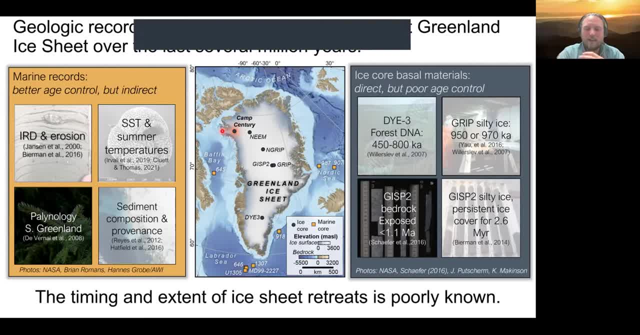 another data point from this uninvestigated subglacial sediment And another reason it's important to go to this part of Greenland is that it's near the margin, So this is one of the parts of the ice sheet that is going to melt earlier than other parts of the ice sheet and raise sea. 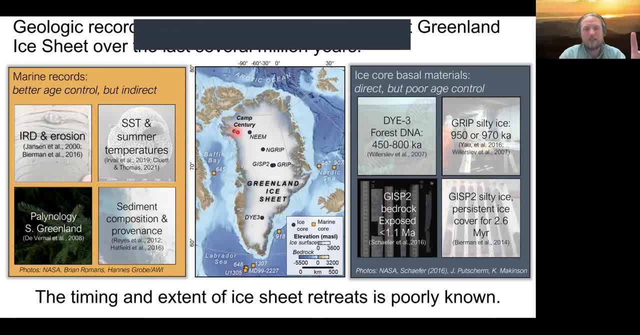 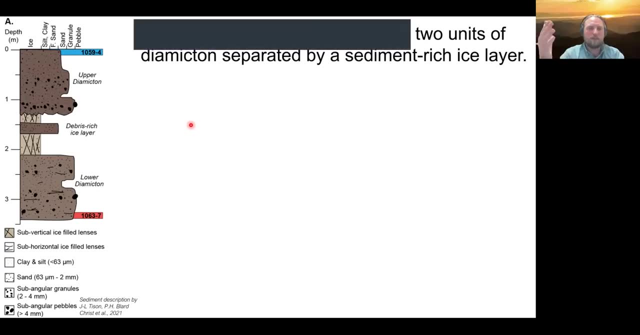 level. So we want to know the ice sheet history of this part of Greenland and the ice sheet sensitivity. So the Camp Century subglacial sediment contains two units of diamictin, which is a poorly sorted mixture of sediment, small grain sizes and lithologies that's separated by a sediment-rich 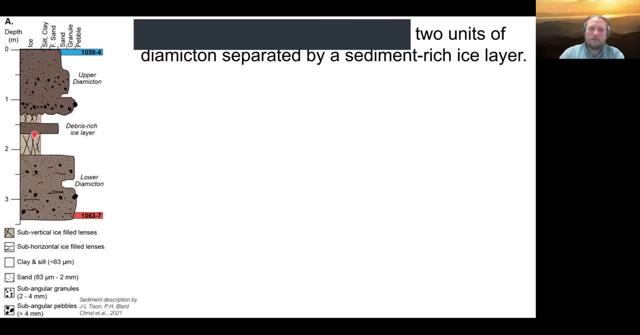 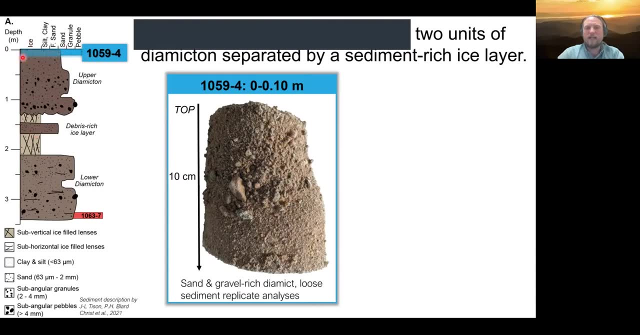 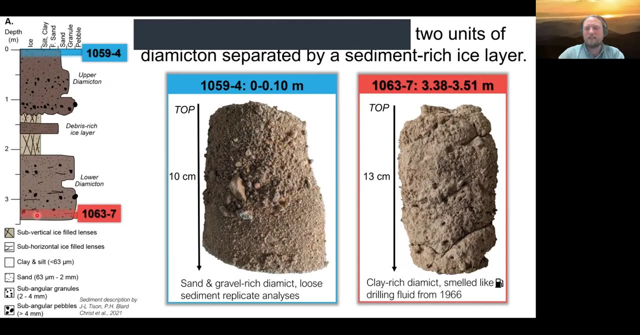 ice layer, And what we have been working on so far is the very uppermost sediment from near the ice sediment interface sample: 10.5.9.. And another piece of sediment from the very bottom of the core- 10.6.3.. 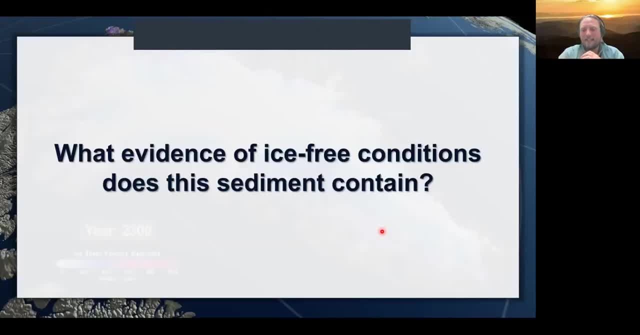 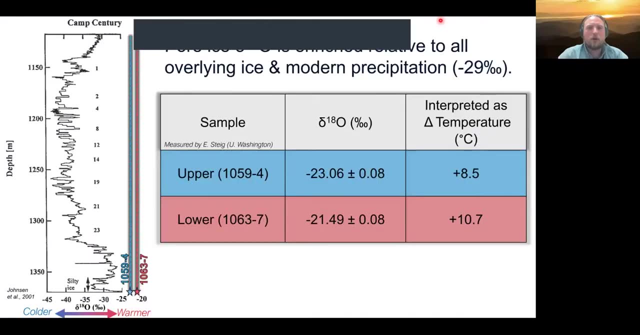 So what evidence of ice-free conditions does this sediment contain? So the first way that we can think about this is by examining the poor ice stable isotopes. And the poor ice stable isotopes are enriched. sorry, there may have been a gray box. 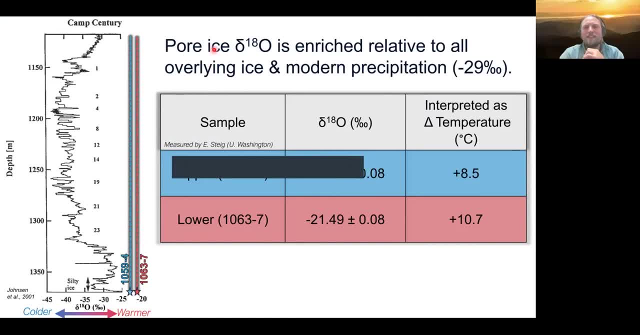 hiding some stuff. sorry about that. The poor ice, delta-018, is enriched relative to all the overlying ice in the ice core and modern precipitation at Camp Century. So modern precipitation is about negative 29 per mil and in the poor ice of this sediment we saw values of 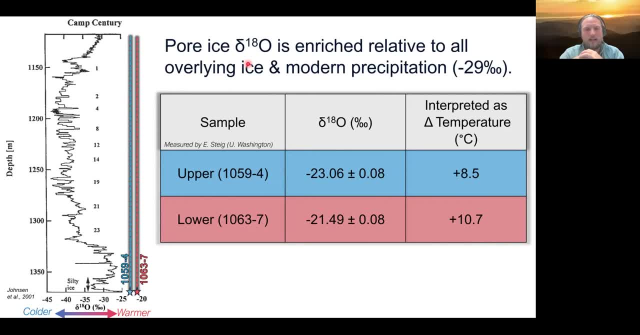 negative 23 and negative 21.5.. And if you plot these values against all of the delo-18 values that are measured in the ice, in the ice core, it's plotted far to the right to more positive numbers, which implies warmer. 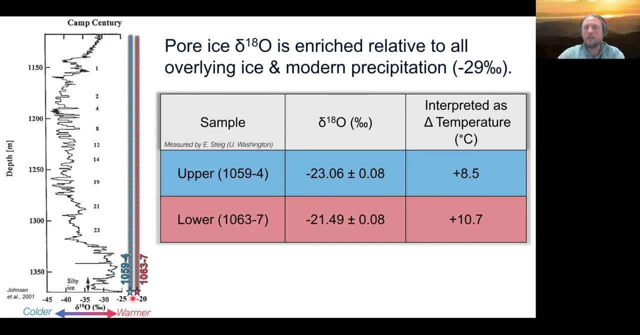 conditions much warmer than anything we see in that ice. So if you were to interpret that just as a temperature change, we would see values that are just way too warm for Camp Century to even to have an ice sheet at it right. It would be impossible to have such one. 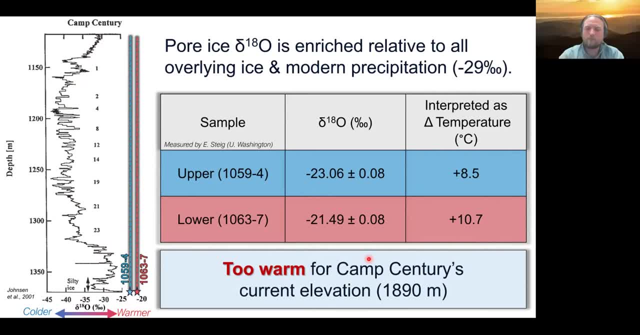 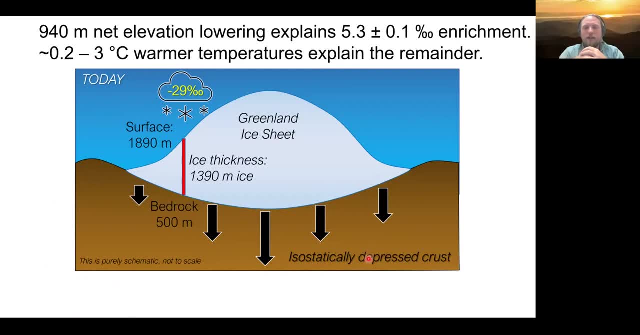 To explain this: enrichment is actually through a net elevation lowering caused by the absence of the ice sheet and isostatic rebound. So I'll walk you through how we get to this. So right now you have precipitation falling at Camp Century with Delo 18 of about negative 29 per mil. 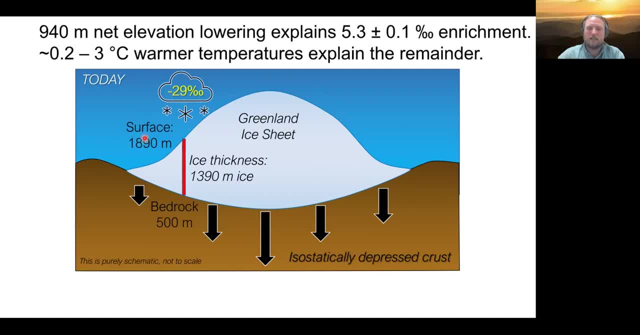 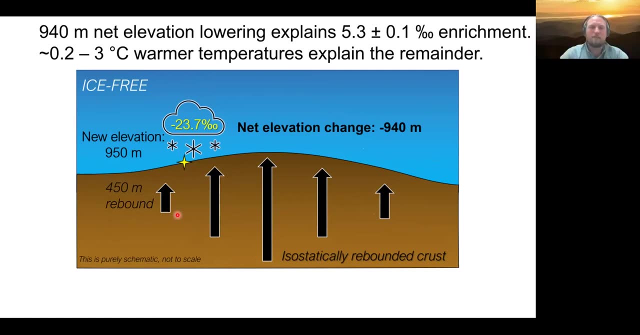 The surface elevation is almost 1900 meters. Beneath that you have a net elevation of about 1400 meters of ice to bedrock at 500 meters. Now, if you removed the ice sheet, the crust would isostatically rebound and cause the bedrock to rise up, So you would end up with a net elevation. 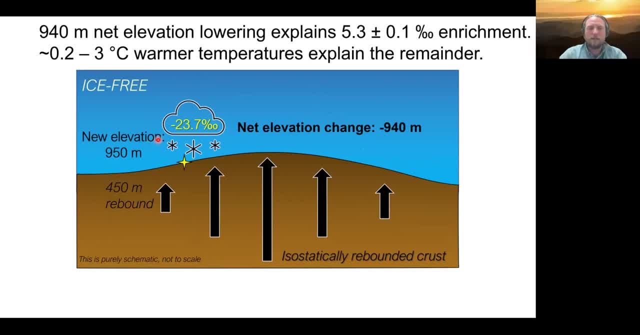 change of 940 meters. That elevation change can account for about 5.3 per mil of the enriched values, And then the remaining enrichment in Delo 18 could be increased by about 5.3 per mil. This is all to say that the poor ice Delo 18 values imply precipitation at lower elevations. 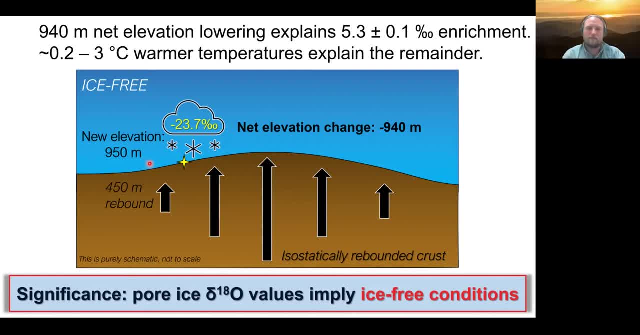 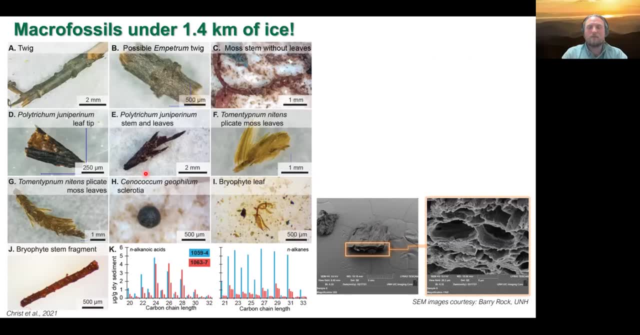 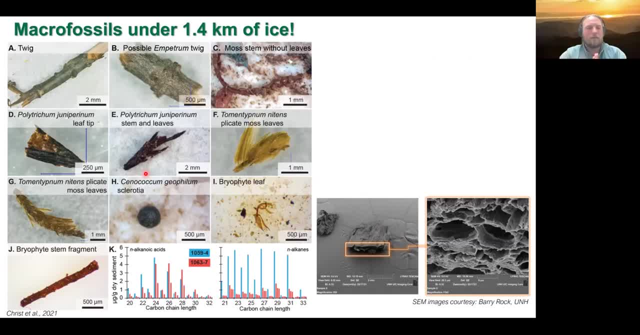 me- it was five days before my phd defense, which had nothing to do with this project at all, um, and we had gotten this sediment and i was a little bit stressed out, as you might understand, ahead of your defense and i was like, do we really need to work on this today? and you know, we're in the lab, we're 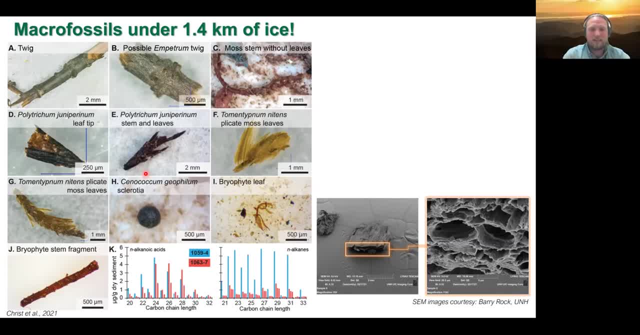 wet sieving this sediment to sort it for other analyses and we see these black specks floating in the rinse water. as we're wet sitting and paul and i um pick up a you know disposable pipe pet and suck up one of those black specks and look at it under the microscope. 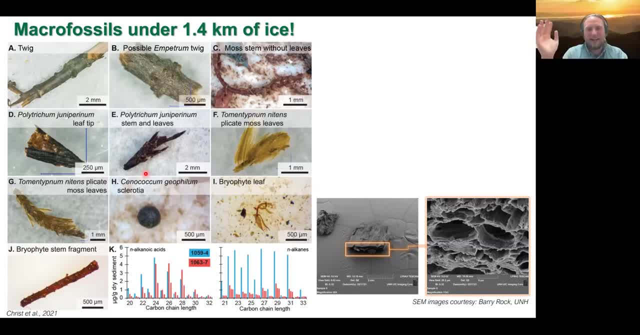 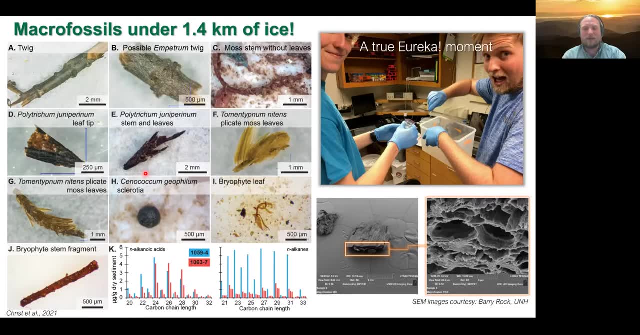 and we just saw a twig and we were. we were like: oh my god, we weren't expecting to find plants in this sediment, we just totally blown away by it and it was one of the most exciting days of science probably in my life and just one of those true eureka moments that i didn't really think had. 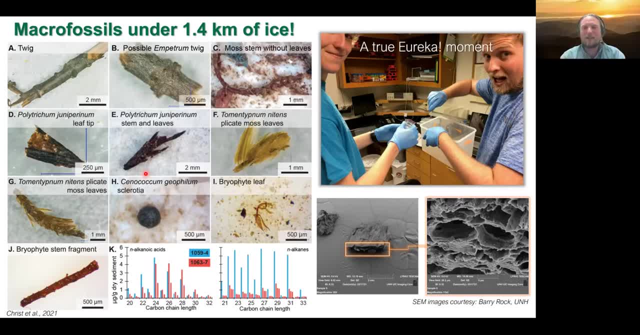 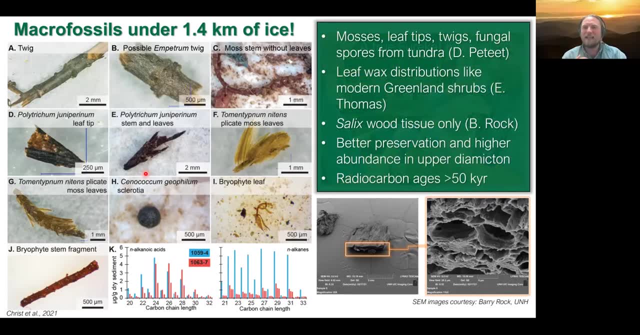 happened, but it did happen. so what we've been learning from, uh, these macro fossils is that we found mosses and leaf, tips and twigs and fungal spores from tundra plants found in ice-free areas of greenland. today we analyzed the leaf wax in the sediments and they have distributions similar to modern greenland shrubs. 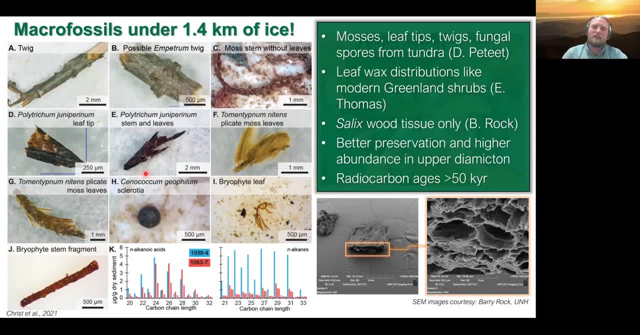 and we recently have examined these pieces of woody tissue under a scanning electron microscope and we've determined that it's mostly arctic willow. we have better preservation of the macro fossils in the upper unit of diamicton, and there's a greater abundance of them too. it took several. 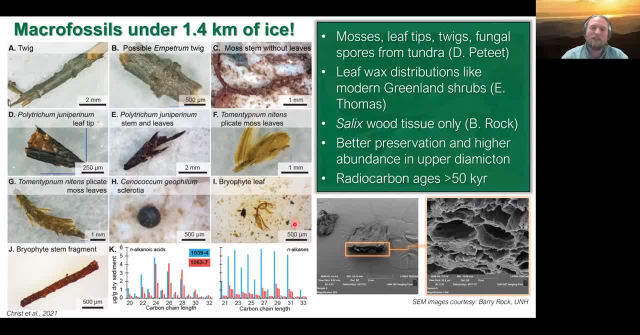 hours to pick through all these different twigs. they really like. i guess like a funny way to think of it is like if you've gone on a hike or a trek and you get a bunch of like twigs and stuff in the bottom of your hiking boot and you like pour it out at the end of the day there's like a bunch of it, right. 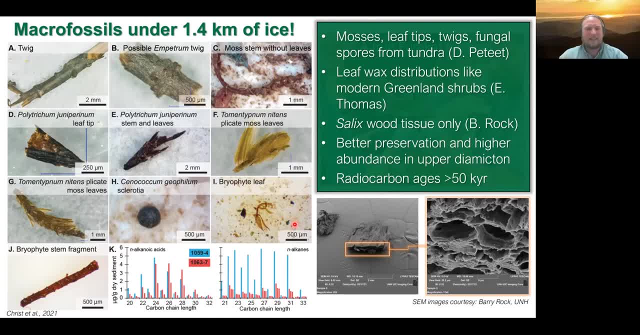 and it kind of looked like that when we were picking this out of the sediment. it just was endless. we wanted to know how old the sediment is, and the first thing that we did was take um one of the twigs and radiocarbon dated and it returned an infinite age, greater than 50 000 years. 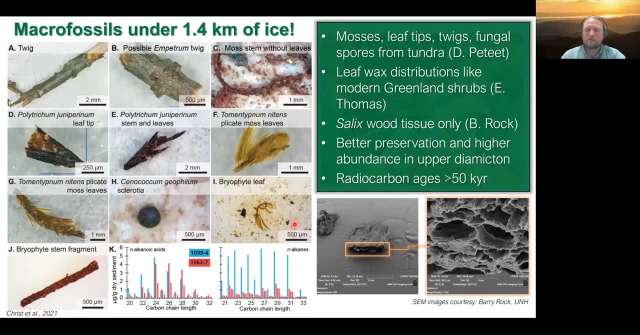 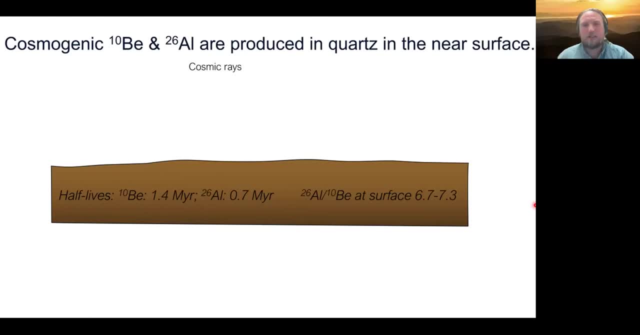 so we knew that this material is quite old, but really the question is: how old is the sediment? so we have a couple of ways that we do this. the first way i'll talk about is using cosgenic nuclides: beryllium 10 and aluminum 26.. these nuclides are produced. 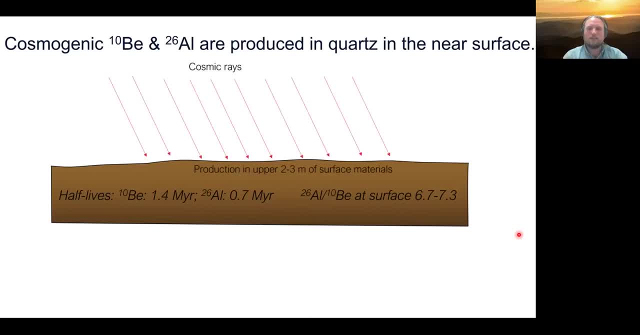 in quartz, in the near upper two to three meters of surface materials in quartz and over time they accumulate in the crystal lattices of quartz. but if you were to um uh produce both aluminum 10 and aluminum, or aluminum 26 and beryllium 10. 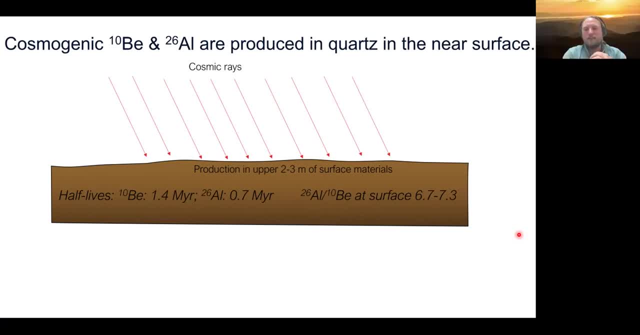 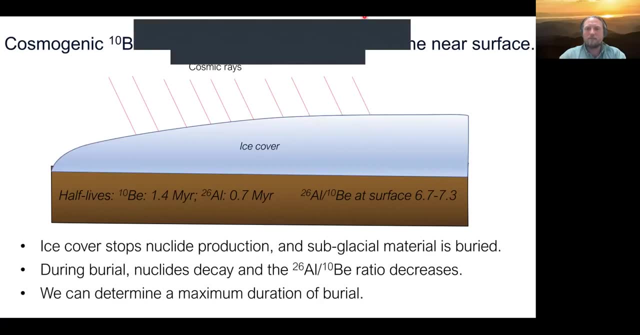 they have a ratio at the surface between 6.7 and 7.3. but if you then advance an ice sheet over that, over the landscape, nuclide production stops, they're hidden from those cosmic rays and then, because they're radionuclides, they begin to decay. 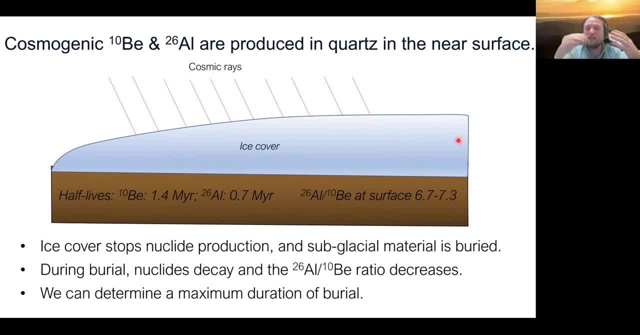 so the total inventory of nuclides decays and the ratio of aluminum beryllium decreases from that initial value of about 7.3. in using that decay rate and the ratio of these two different nuclides we can determine the maximum duration of burial in sediments. so that's one way that we did this. 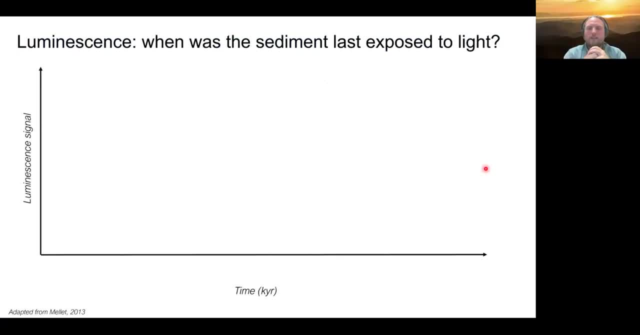 now, the other way that we can determine the age of these sediments is using luminescence dating, which essentially answers the question: when was the sediment last exposed to light? I'm not a luminescence expert, but I'm going to give you just an overview of how this 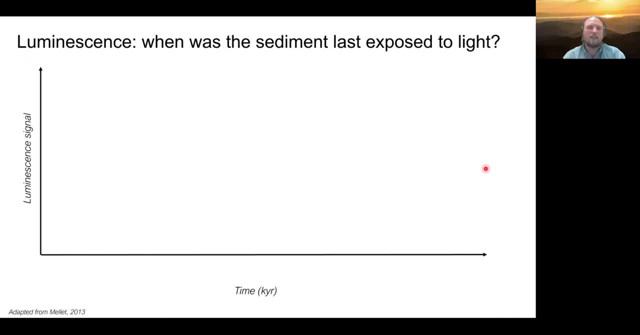 works because it was new to me. So luminescence dating relies on the idea that when sediments are buried beneath the surface and hidden from sunlight, the background radiation in sediments and soils will excite electrons that will fill in the crystal lattices, the impurities in the 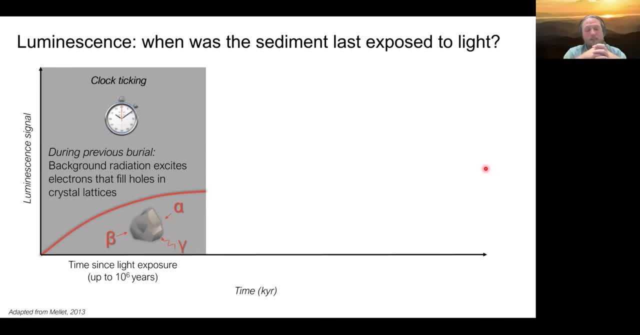 crystal lattices in different minerals like quartz and feldspar, And over time that will accumulate a luminescent signal. But if you expose that sediment to sunlight it bleaches the electrons out, So you lose the luminescent signal. If you bury it again, that same. 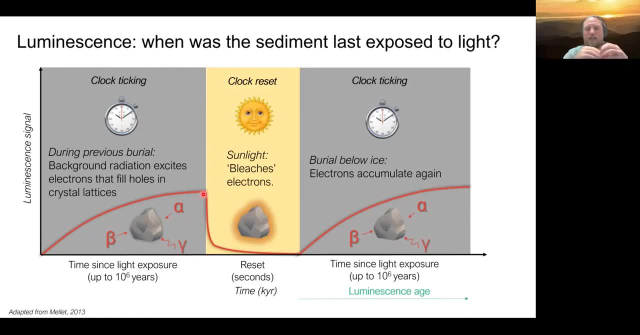 luminescence will accumulate a luminescent signal. So when you bury it again, that same luminescence signal will accumulate a luminescence signal. So when you bury it again, that same idea happens again. You accumulate those electrons in the holes in the crystal lattices. 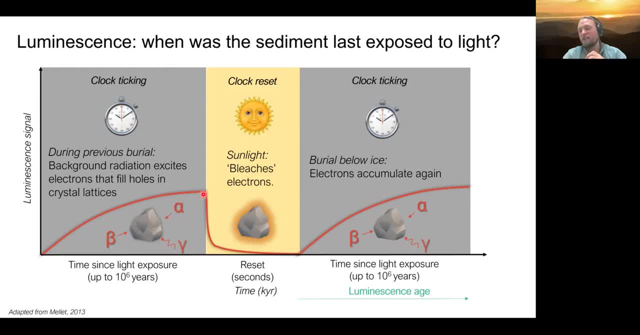 from the background radiation. But in some minerals like feldspar, you actually have a little bit of fading. Some of those electrons are released out, And then, geologists, we have to sample this in the dark So you can't expose the sediment to sunlight, Otherwise you're going. 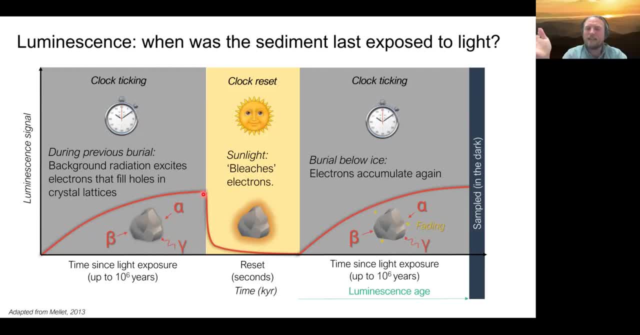 to reset your clock Now. if this didn't make sense to you, you can think about wearing dirty clothes. If you just wore the same shirt every day for a month, it would accumulate a stinkiness index right A stinkiness signal. But if you put it in the washer it's going to. 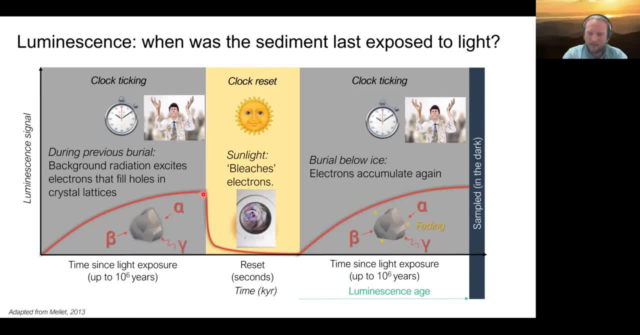 not be stinky after about a few minutes. Then if you wear that same shirt again for a month, it's going to accumulate that stinky signal. That's kind of the same idea with luminescence dating. So what are the ages that we get with these two different methods? I'll start with the lower. 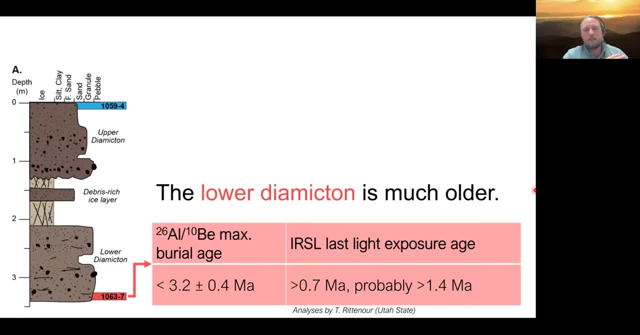 diamicton, which is much older. Using aluminum beryllium burial dating, we know that it has been buried no more than 3.2 plus or minus 0.4 million years, With the infrared luminescence dating on feldspars. the last light exposure was before 0.7 million years ago, but more likely before 1.4. 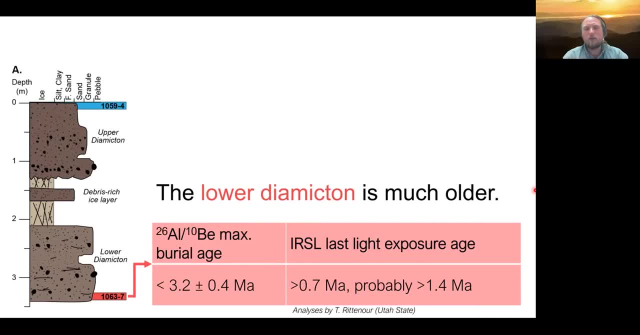 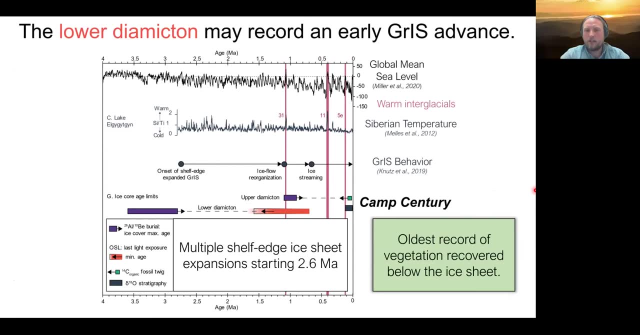 million years ago. This lower diamicton may record an early advance of the green lanai sheet, So in this figure I am showing the last four million years with some different paleoclimate indicators that are relevant to Camp Century, global mean sea level and Siberian. 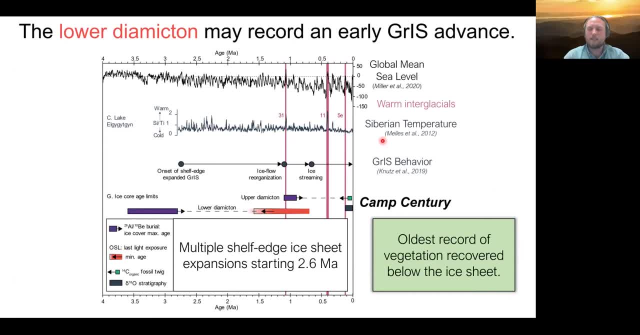 temperature at the Lake Yee sediment core. And so if we place these age constraints of the lower diamicton from Camp Century, we see that it is correlative with the very early beginnings of the fully expanded green lanai sheet, Starting about 2.6 million years ago, The presence of the tundra twigs and leaf tips and mosses in this. 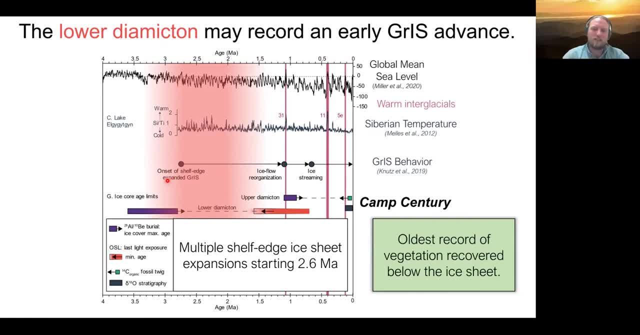 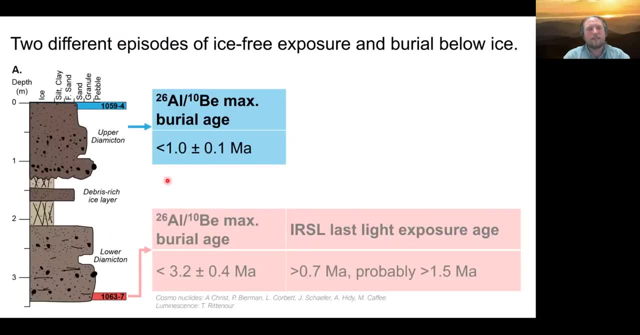 set a, the oldest record of vegetation recovered below the ice sheet so far. Now, what about the upper sediment? Well, the upper sediment has very different age constraints. So that tells us there are two different episodes of ice: free exposure and burial below ice. 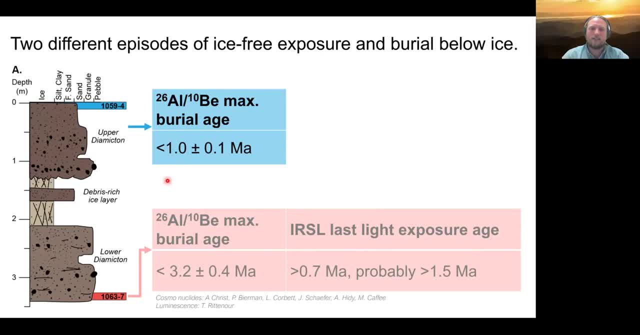 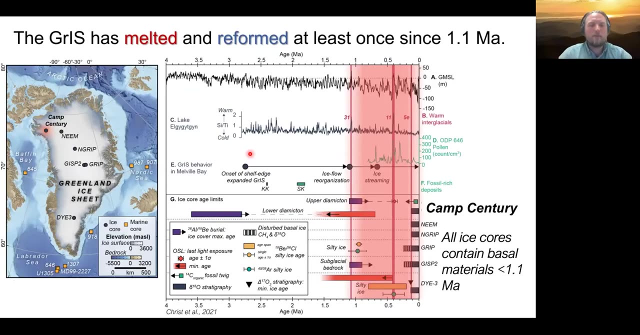 I'll start with just two, discussing the cosgenic nuclide constraints on the upper diamicton, which requires exposure within the last 1.0 to plus or minus 0.1 million years. This new age constraint gives us quite a bit of confidence that the Greenland ice sheet 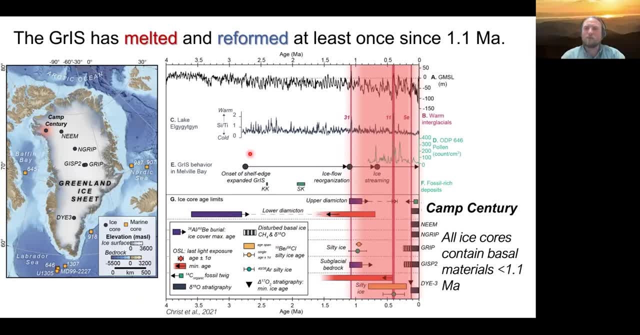 has melted and reformed at least once in the last 1.1 million years, because all of the ice core basal materials, from the interior and to the south, they're all younger than a million years old. So there is nothing at the bottom of these ice cores that tell us that the ice has been 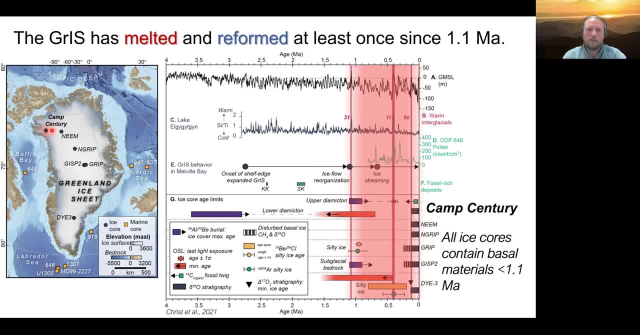 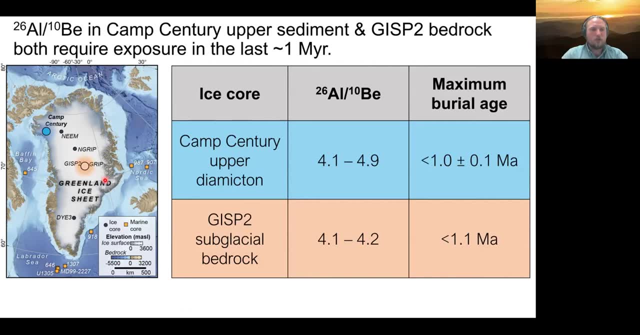 present for longer than a million years. And then I want to focus in on Camp Century versus GISP-2.. And GISP-2 is in the very interior of the ice sheet, just near the summit, whereas Camp Century is near the margin. 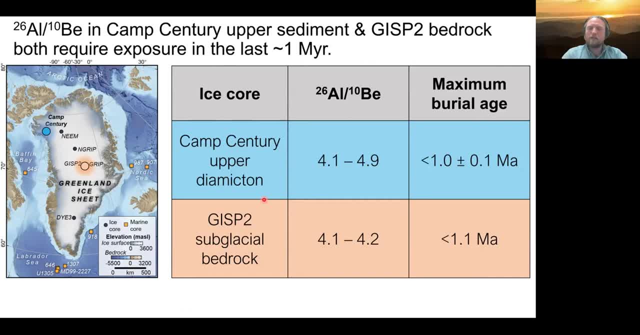 Now these two different archives, the subglacial sediment and the subglacial bedrock, have similar aluminum-beryllium ratios and that suggests a similar burial history. But the maximum burial age requiring exposure in the last million years at both sites is: 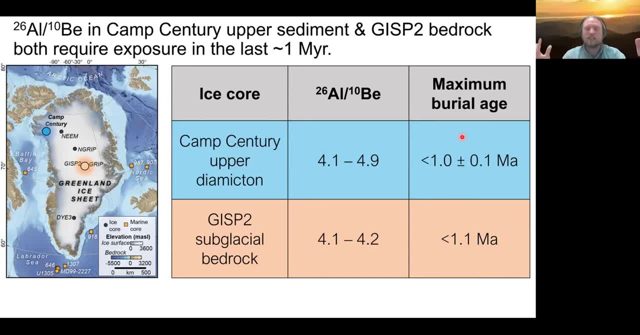 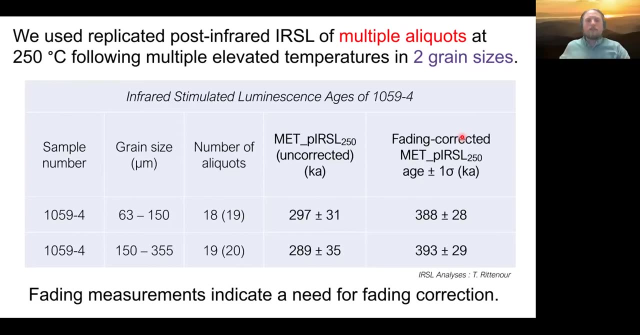 really great evidence that this ice sheet has disappeared in that time frame, suggesting a similar history of ice cover. between the margins, Now we have better age constraints on the upper Diamicton because we were able to get some infrared luminescence dates that we've been collecting or measuring over the last. 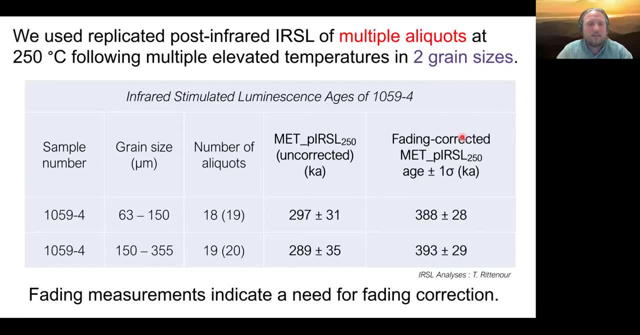 few months or so, with the help of Tammy Rittenhour at Utah State, And so we tried to get a robust data set from the sediment. So we used multiple aliquots, meaning analyzed multiple grains of feldspar In two different grain sizes of the same sample. 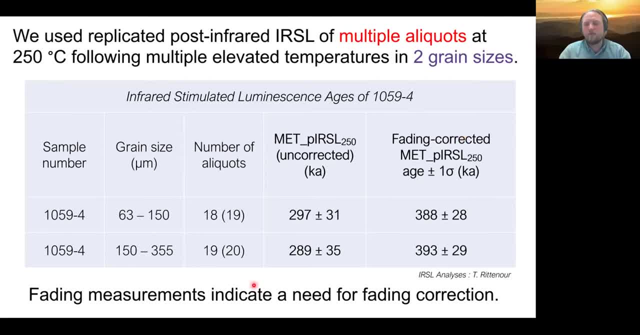 So ultimately we have nearly 40 measurements on grains that produce infrared luminescence ages of about 290,000 years. Now, if you remember, I mentioned that with feldspars you have to correct for fading, And the fading measurements we collected suggest that if you correct for fading, you're going. 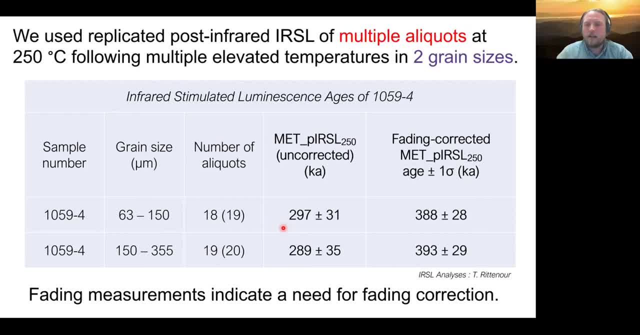 to be able to correct for fading. So if you correct for fading, you're going to be able to correct for fading. So if you correct for fading, you're going to be able to correct for fading. We get um RSL ages of about 391, plus or minus 28,000 years ago. 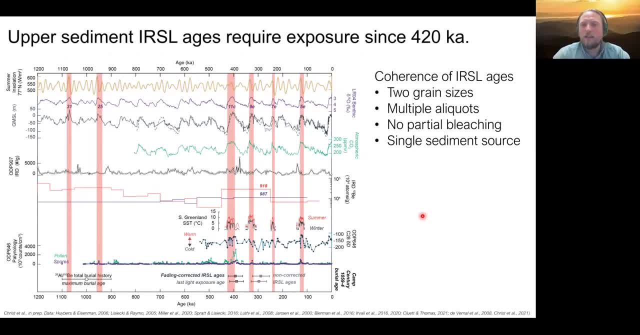 These upper sediment luminescence ages require exposure and thus an ice-free event in the last 420,000 years, And we think that these RSL ages are a robust dataset because we have coherent ages and two grain sizes with multiple aliquots- don't see any evidence of partial bleaching from exposure to sunlight, otherwise we'd see much. 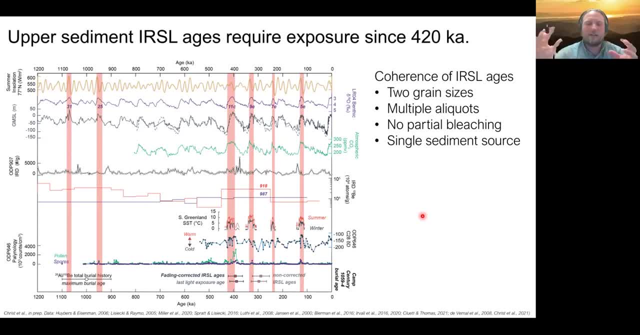 larger spread in the data and we don't think that this sediment is a mixture of sediments with different exposure histories because the data are so coherent. What does this mean in terms of paleoclimate? So, if we place these age constraints from the RSL ages against 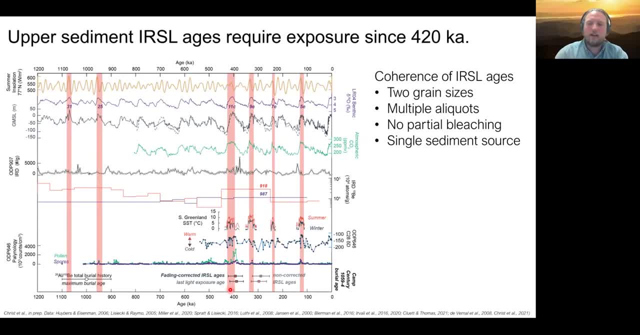 different paleoclimate records. without a fading correction, these ages fall into the MIS VIII glacial period. Now, that doesn't really make sense for an ice-free event to occur during the middle of a glacial period. So if we then consider the fading corrected ages, they date to just after. 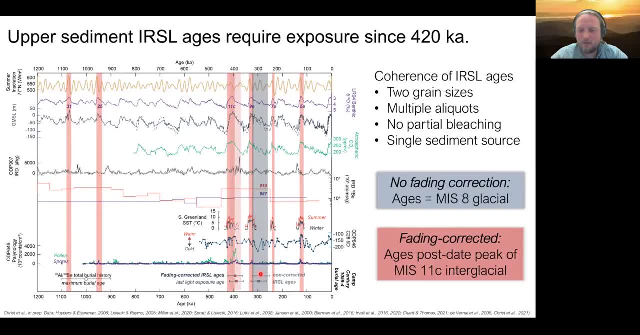 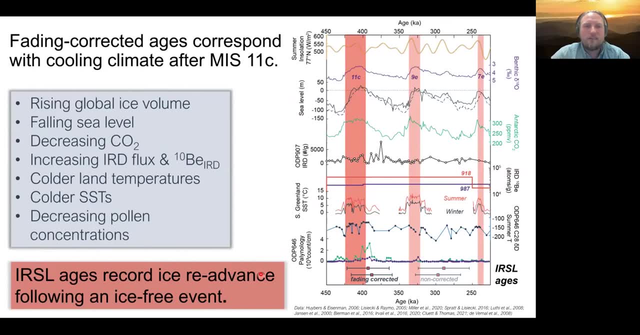 the peak of the MIS XI C interglacial. So So the fading corrected ages from the upper Diamicton correspond with a cooling climate after MIS 11c. I've zoomed in here on a time span of about between 450 to 250,000 years ago. 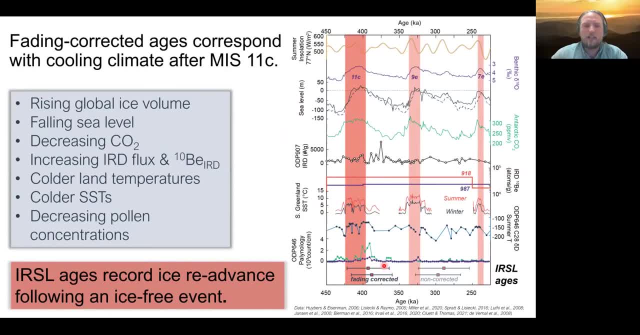 And just to direct your eyes, here is the fading corrected age, And we can see that these fading corrected ages coincide with growing global ice volume from the benthic del 18 stack, falling global sea level, declining carbon dioxide, an increase in ice rafted debris flux as the ice sheet got. 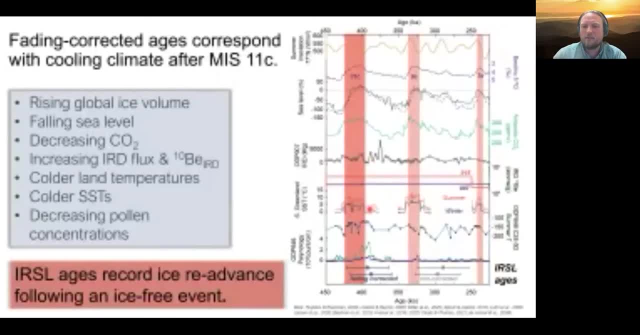 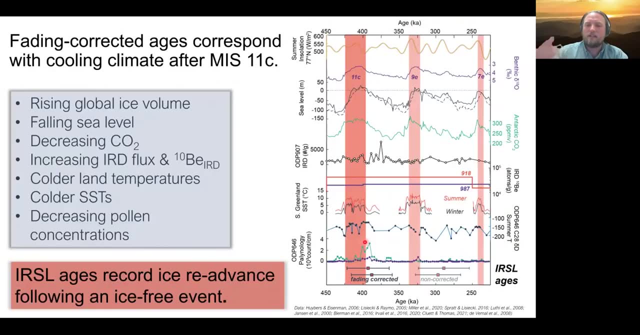 larger, as well as cooling sea surface temperatures, land temperatures and the decline in pollen concentrations into the Labrador Sea south of Greenland, suggesting that the ice sheet was getting bigger. So these infrared luminescence ages actually record the re-advance of the Greenland. 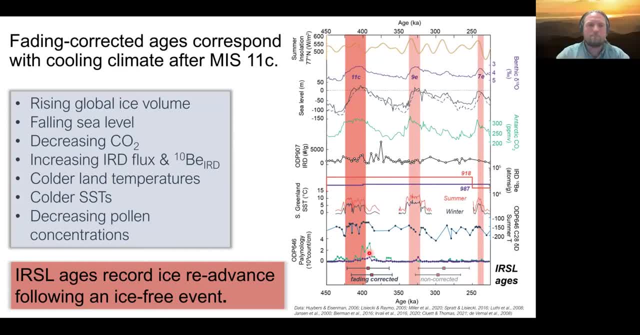 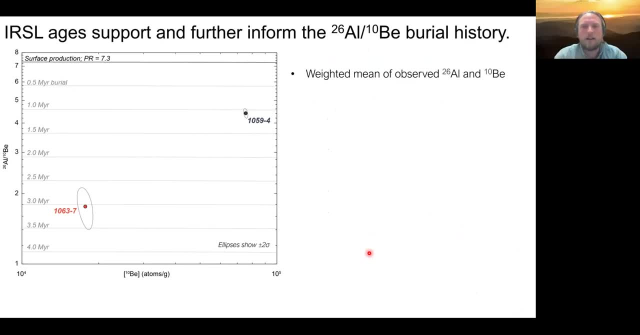 ice sheet and burial of this sediment. We can use the infrared luminescence dating to support and further inform our cosogenic nuclide burial history. It's a little bit of a complicated plot, but I'm going to try and walk you through it. 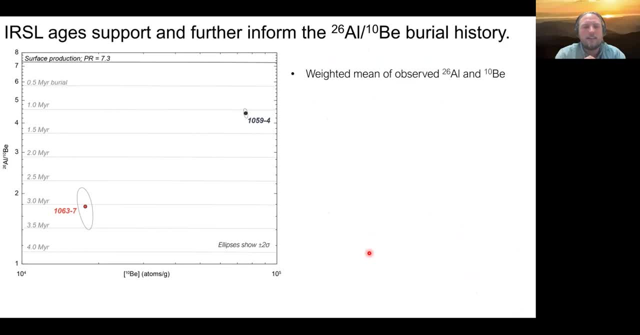 So this is the two isotope diagram that we use in cosogenic nuclides. Over time, on the x-axis, if you expose sediment, it's going to accumulate more beryllium-10.. And if it's at the surface. but if you bury that sediment, 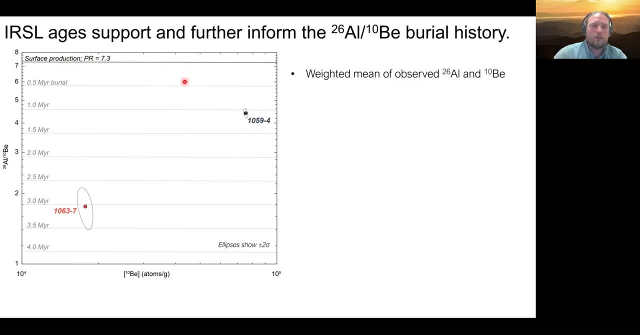 those nuclides begin to decay and the ratio between them decreases. So these are the measured values that we got for the upper sediment and lower sediment. We can correct these for the burial time of 390,000 years to get an idea of what the burial history was at the end. 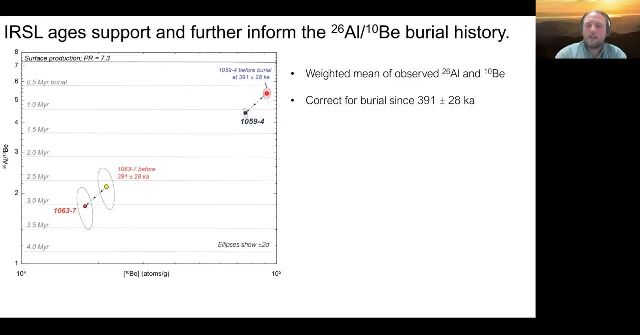 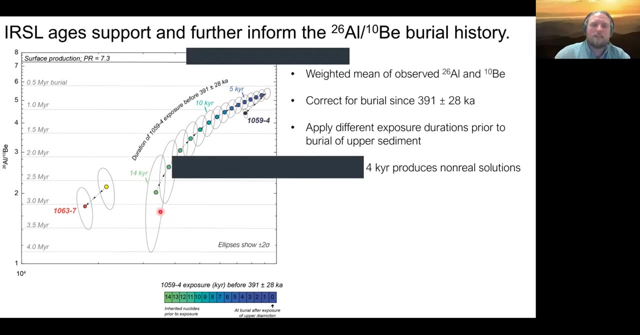 of the last. We can then simulate exposure simulations onto those sediments to tell us how long they could have been exposed. So you cannot expose this sediment, the upper sediment, for more than 14,000 years or you end up with an initial burial history that 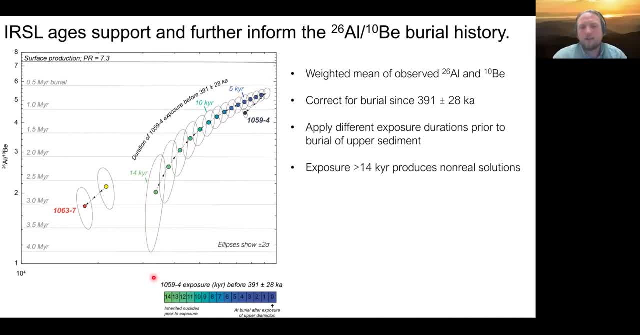 suggests negative burial, which is impossible. So what this means, And then I'll talk about this in a second- but we can also correct for additional burial of that lower sediment which we presume was not exposed during that last event. But what I want to take away from this plot, 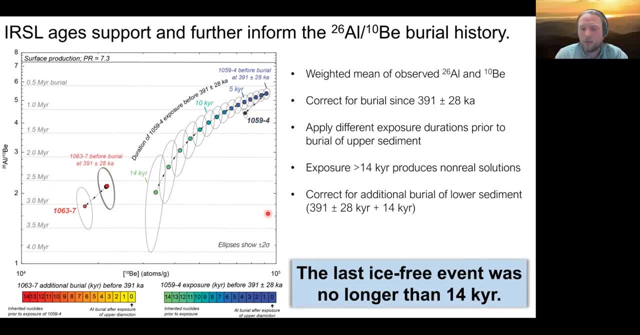 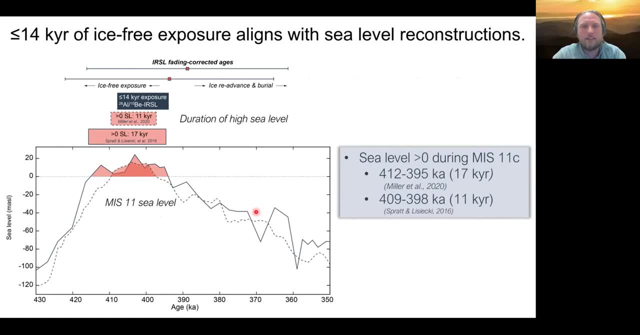 is that that last ice-free event was no longer than 14,000 years. Less than 14,000 years of ice-free exposure in northwest Greenland aligns with sea-level reconstructions during MIS-11-C. So we have, So we have. 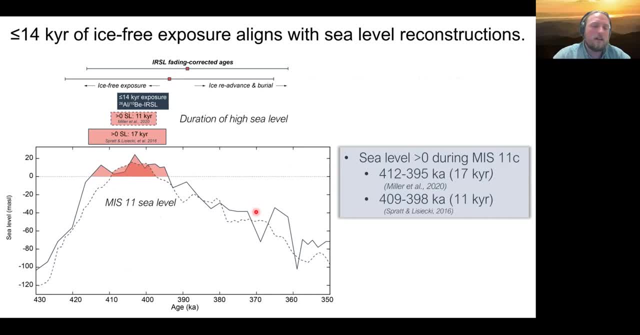 We have two different data sets that I'm just comparing this to that are based off of the benthic DELA-18 stack, which both suggest that sea level was higher than present between 11,000 to 17,000 years of duration during MIS-11-C. 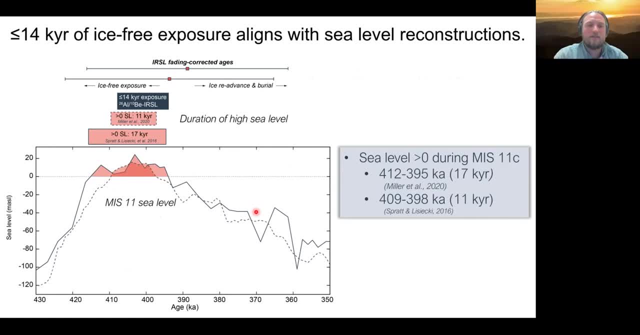 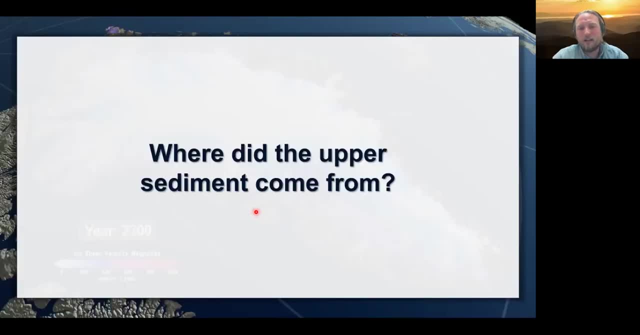 And so that 14,000 years of exposure at Camp Century is consistent with those durations. Now we need to know: where did this upper sediment come from? And I want to go back to, And I want to go back to, And I want to go back to. 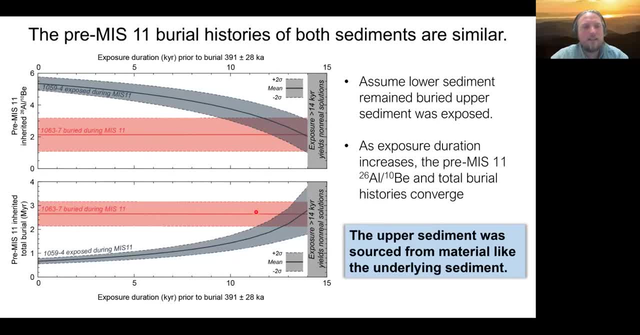 Our burial history again And see if you correct that upper sediment for buried for exposure during MIS-11 for up to 14,000 years and calculate what the incoming aluminum-beryllium ratio is and compare it to the lower sediment, you see that they're very similar. which? 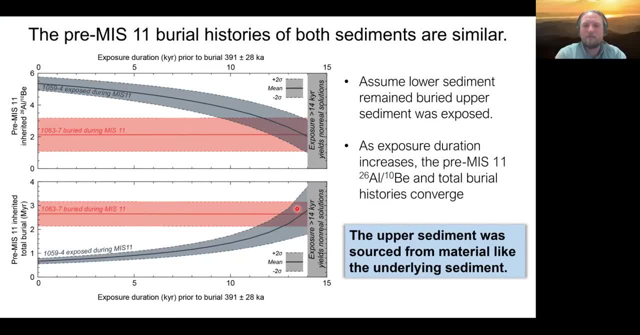 implies that they had a similar burial history to begin with And that suggests to us that the upper sediment was sourced from material that was like the underlying sediment. And that suggests to us that the upper sediment was sourced from material that was like the underlying sediment. 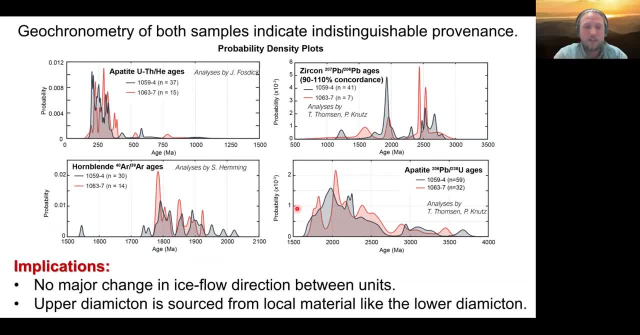 We did a series of different geochronometry analyses on both sediments And we see across different geochronometers that they have indistinguishable provenance, meaning that there was no major change in ice flow direction between the units, And it also suggests that that upper diameter 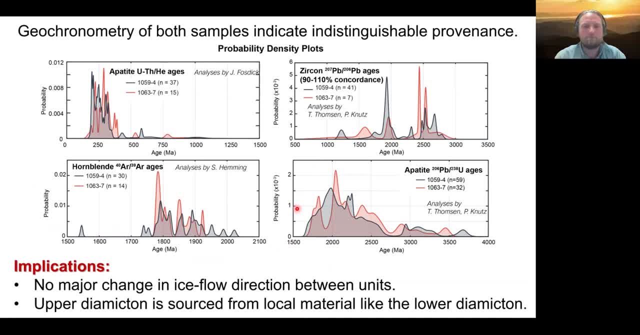 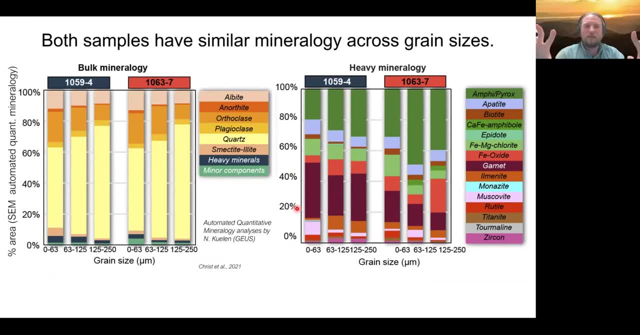 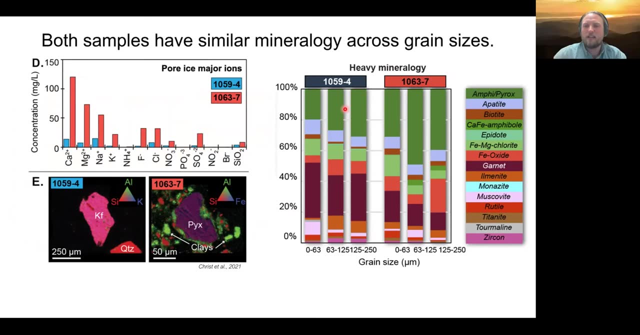 material is similar to the lower diameter. Both of those sediment samples have really similar mineralogy, especially the bulk mineralogy, But they are slightly different in the heavy mineralogy between amphiboles and pyroxenes and garnets And we think this may be reflective. 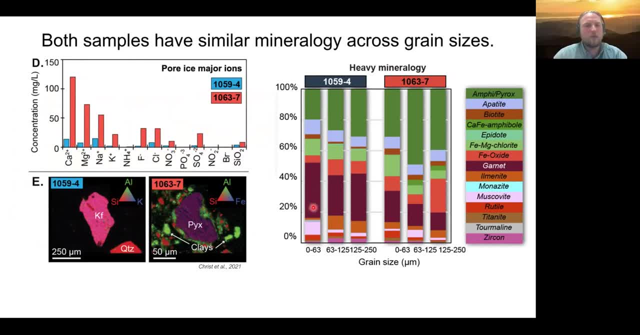 of a slightly different weathering history between the two units, which we've already observed in the porous ion concentrations and weathering clay grain coatings on each sediment. that suggests that they had a different weathering history. So it suggests that the upper sediment may have been weathered more intensively. 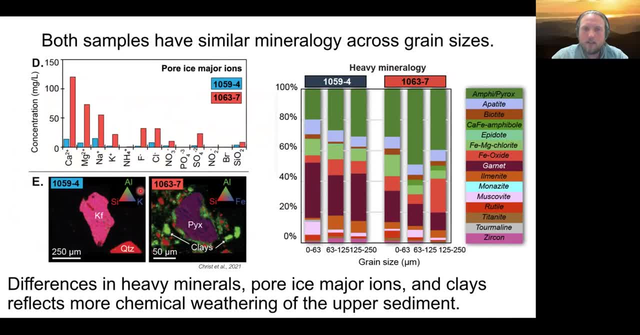 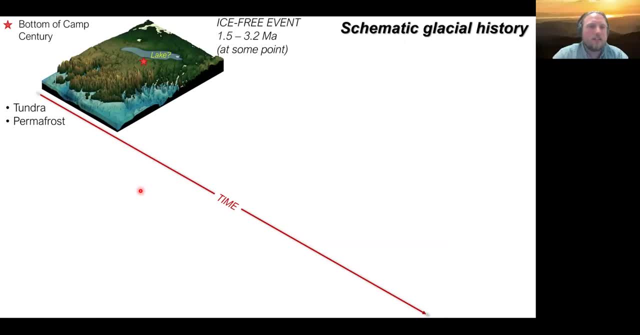 than the lower sediment. So I just want to put this all together so we have some sort of schematic of what happened. This is showing just schematically the Greenland landscape and what we think was happening. We have an initial ice-free event where we have tundra growing sometime in the early Pleistocene. 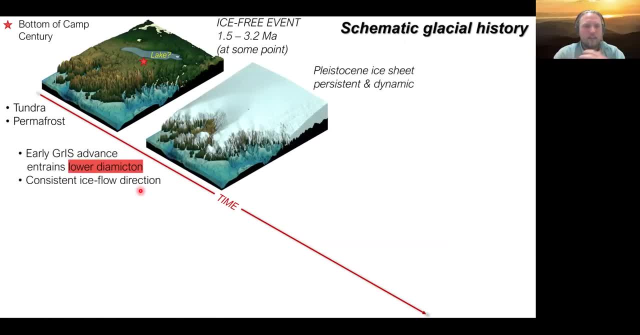 We have ice cover during much of the Pleistocene that entrains the lower diamicton beneath the ice sheet with consistent ice flow direction, And then we have an ice-free event during MIS 11C camp century with duration of no more than 14,000 years. 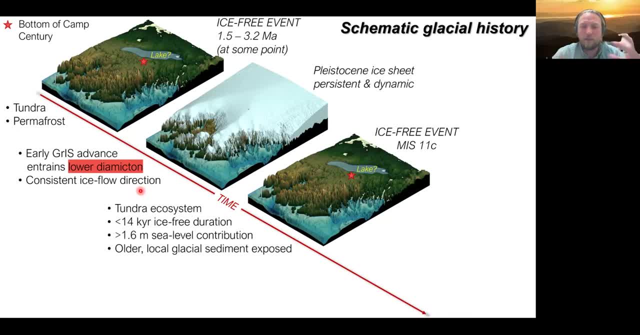 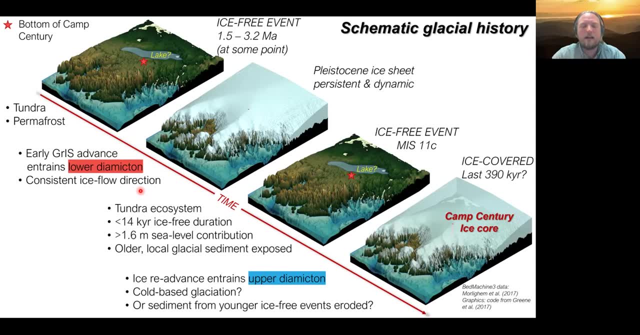 with older local glacial sediment exposed and weathered, And then a re-advance of the ice sheet that entrained that upper diamicton. And then you know, the Camp Century ice core is collected and recovered, you know, in the last 60 years. So one. I'll wrap it up soon here, But 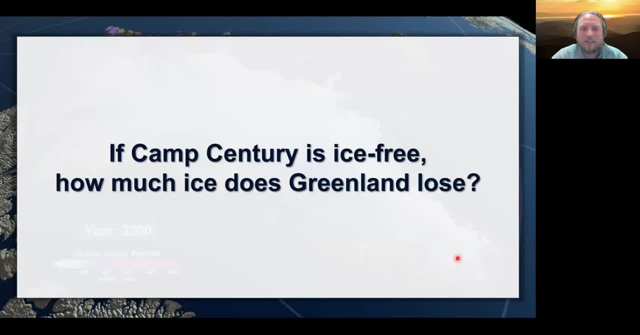 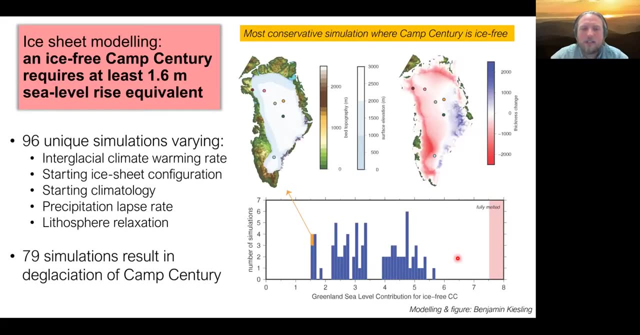 if Camp Century is ice free, how much ice does Greenland have to lose? Benjamin Kiesling has been doing some ice sheet modeling work to figure this out And he ran 96 unique simulations varying a variety of parameters, And he found that, in order to 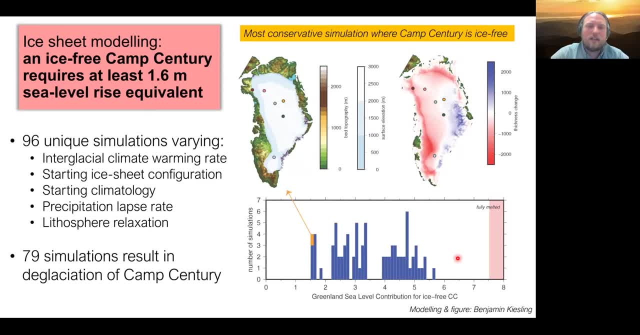 expose Camp Century. the configurations of the Greenland ice sheet require a contribution of at least 1.6 meters of sea level rise, So this is the most conservative configuration of the Greenland ice sheet that allows Camp Century to just barely be ice free And that 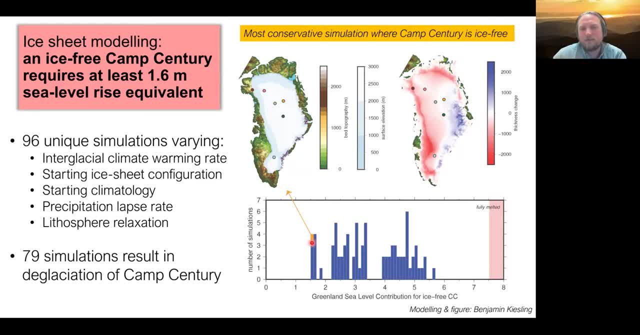 requires a lot of work, And so he found that, in order to expose Camp Century, the configurations of the Greenland ice sheet require at least 1.6 meters of sea level rise. It could be more, and there's a lot of spread in the data, but this is a hard bottom for that contribution. 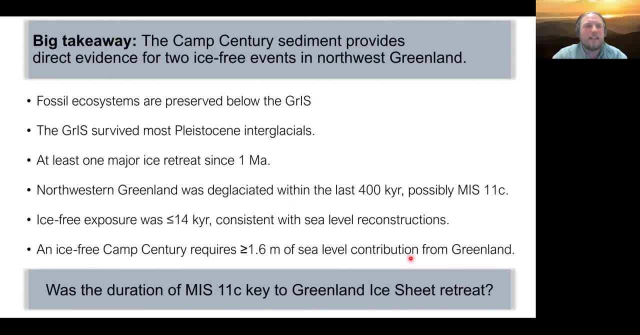 So big takeaway here is that the Camp Century sediment provides direct evidence for two ice free events. in northwest Greenland We have preservation of fossil ecosystems beneath the Greenland ice sheet. It seems that the Greenland ice sheet persisted through most 600 years, So, for example, there's a lot of ice in the Grail We can observe in that. 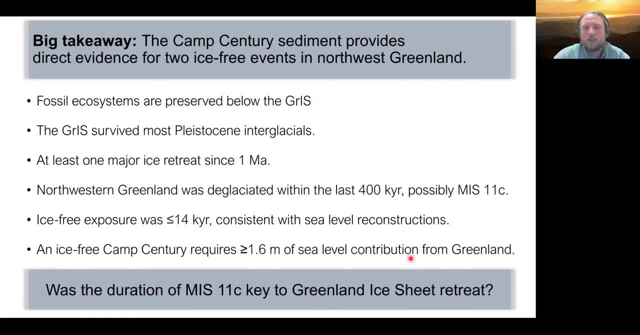 dumpster, an avalanche of ice and a huge amount of land, And that's probably the only possibility. So that's the next thing I just seen. So a few years ago, northwestern Greenland was deglaciated within the last 400,000 years. 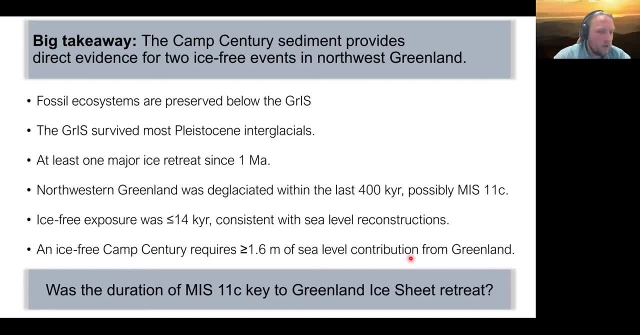 possibly during MIS 11, during an event that was no more than 14,000 years long, And an order for Camp Century to be ice free requires at least 1.6 meters of sea level. contribution from Greenland. I just want to finish with one idea. here is: you know why is MIS 11's? 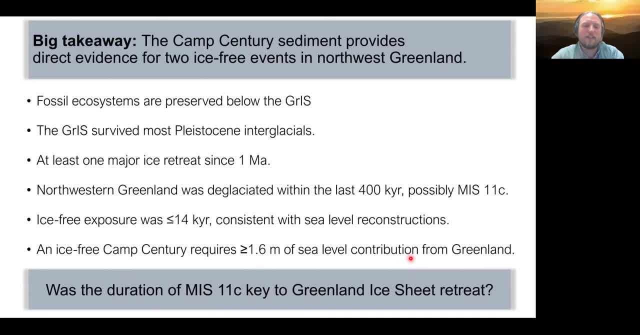 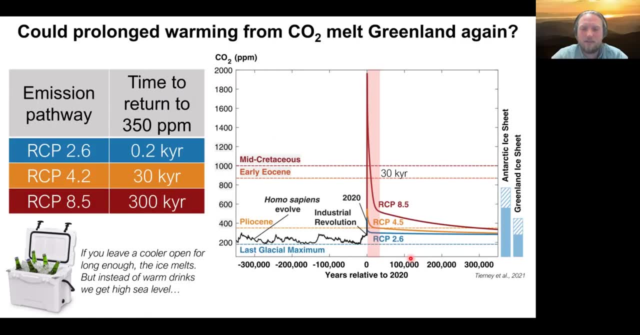 11 such a special interglacial or warm interglacial that had such high sea level And it was very long. it was 30,000 years long. So I just want to think more forward here- is if the long duration of MIS-11c. 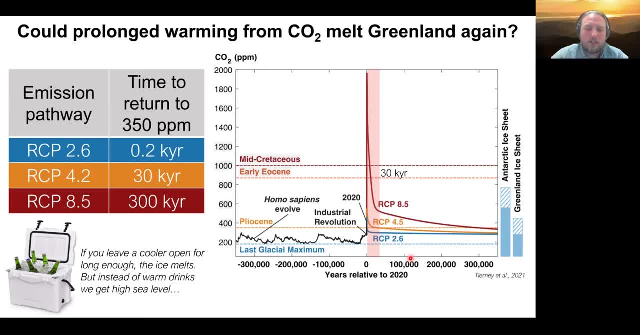 30,000 years was long enough to melt a large portion of the Greenland ice sheet. what's going to happen if we continue to pump carbon dioxide into the atmosphere? and it has a long resonance time. So this is a recent review paper by Jess Tierney that was out earlier this year. 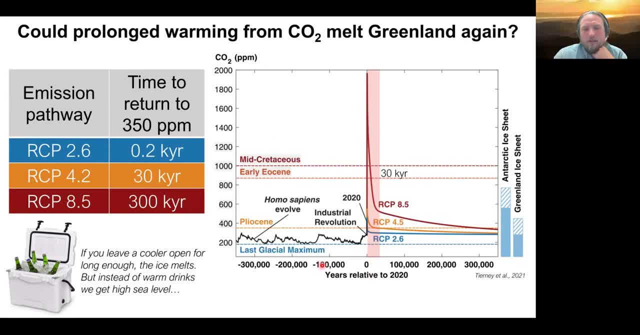 and I really like this graph where she shows how much time it will take to reduce carbon dioxide concentrations back to 350 parts per million. And even under, you know the moderate RCP emission scenario 4.5,, it's going to take 30,000 years to get back to 350 parts per million. 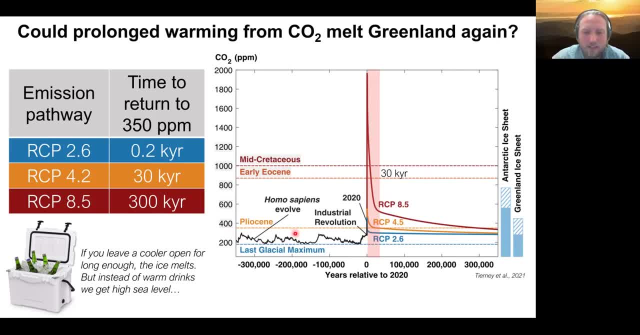 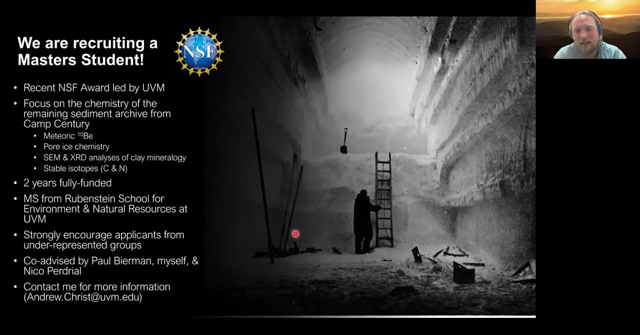 So if 30,000 years was long enough to melt northwestern Greenland during MIS-11, you know what does that mean if we continue to warm the climate for very long periods of time. So, last thing, we just got funded to do the remaining archive. 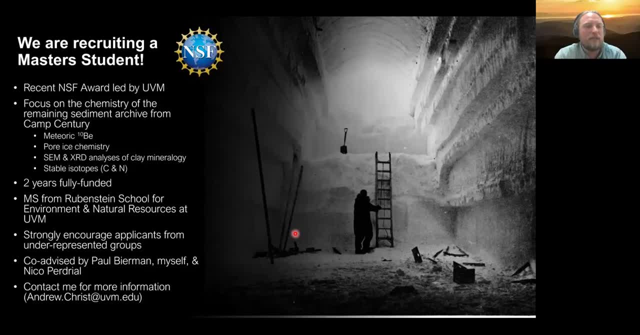 analyze the remaining archive of the sediment and we are recruiting a master student to dive into some of the chemistry about the soil development as well as weathering history, And you can contact me for more information about that. So sorry if I went a little bit over, but thanks so much for all. 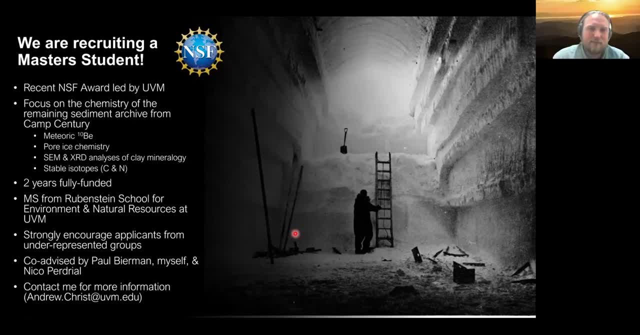 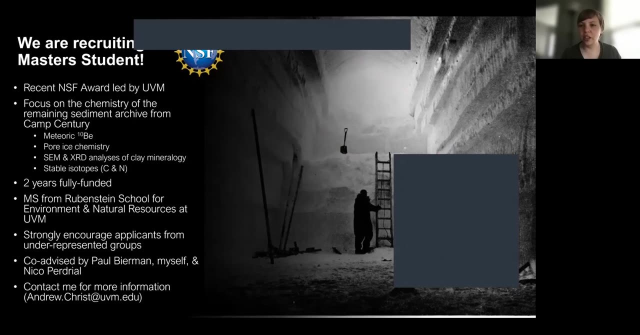 for you all coming today and I look forward to chatting with you. Hey, thanks, So yeah, so just a reminder that you can send your questions via the chat to: I got it wrong before. It's Natasha who's the questions at Paleo perks this week. 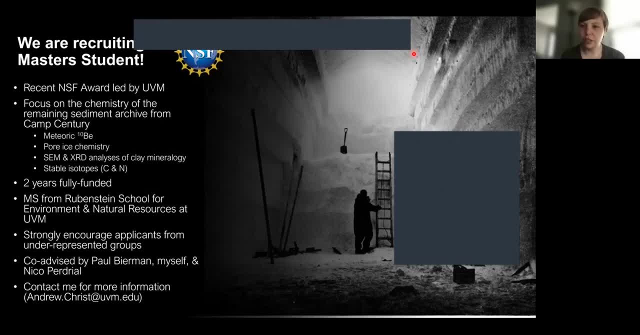 So if you have any questions that you want to send, you can do that now or again. raise your hand if you'd rather try that way, And we've already got a few coming in. So let me put it into the chat really quick. 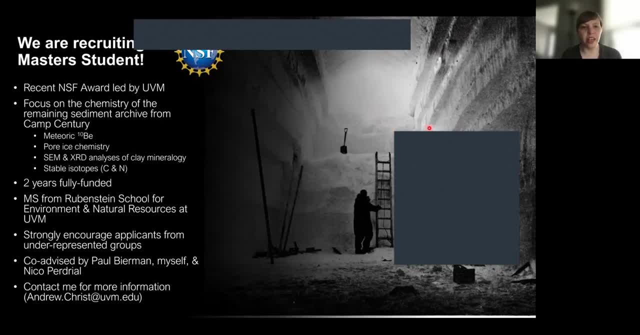 So it says this data set is so cool and it's really impressive. how many aspects of Greenland. How do you know whether the sediments slash macrofossils are from Camp Century's specific location, or do you think they could have been moved or dragged at the base of? 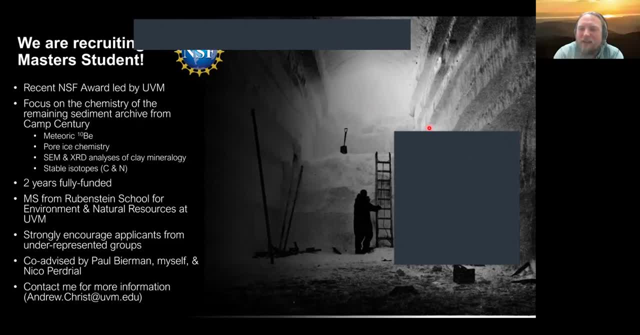 the ice sheet? Good question. Yeah, the origin or the location of the origin of these sediments is something that is difficult to answer, but I have a couple of ideas about this. There's one line of evidence that suggests from geophysical measurements, radar measurements over 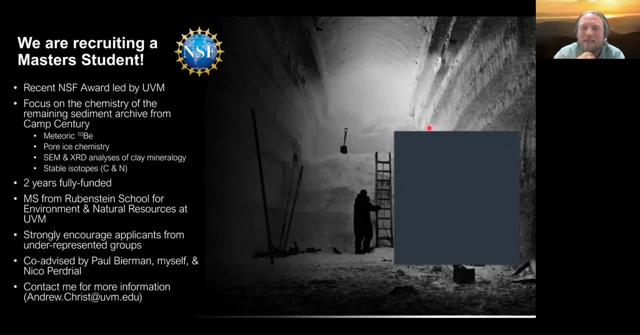 the Greenland ice sheet that there is a large lake basin in this part of northwestern Greenland that is hidden beneath the surface of the ice sheet. It's an extensional normal fault valley that has filled in with sediment and it's unclear if it becomes a lake during ice-free events. 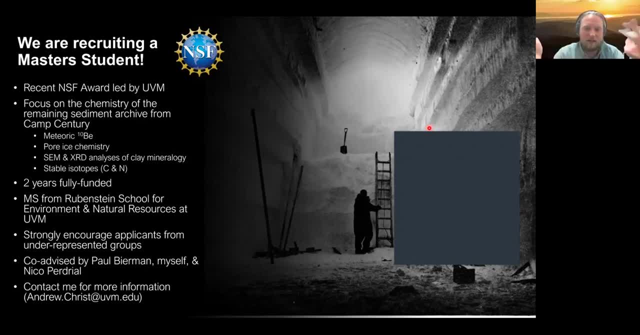 So it's possible that you know this was kind of the environment that was there. It was this tundra ecosystem with ponds and lakes scattered across the landscape, kind of like we see in ice-free areas in Greenland today, at least in the more sub-corridor regions. I think that 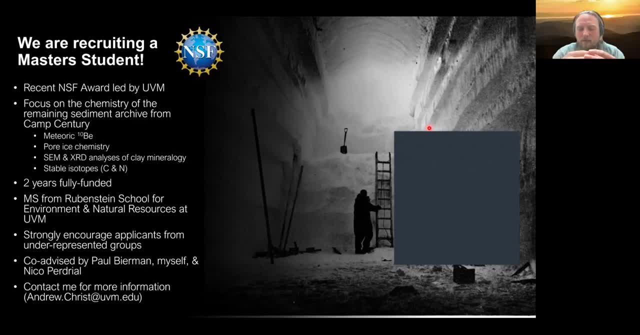 you know, they probably moved locally because the lower sediment and upper sediment have so many similarities in terms of their burial history. initial burial history geochronometry, You know that suggests to me that it is more or less local. Of course it may have been transported a short distance. 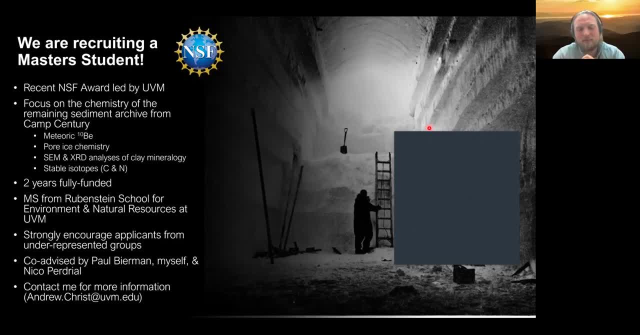 and then another reason, one more reason I think that they're relatively local to here- is that the preservation of the fossils in the upper Diamcton is it just seems too well-preserved to have been transported a long distance, because I would imagine that long-transport distance is. 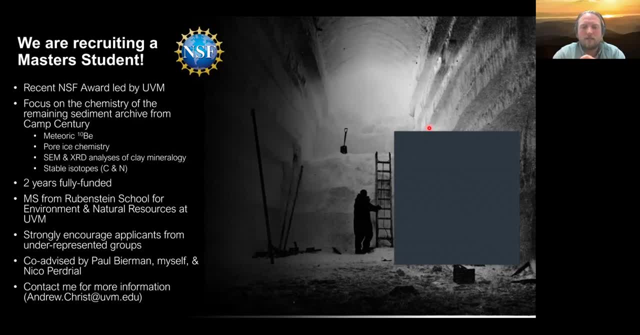 distances under flowing ice or warm based ice would destroy a lot of that material. So I think that it's mostly local and that actually that much of the time it's been beneath the ice sheet it's been cold based glaciation, which is not erosive. 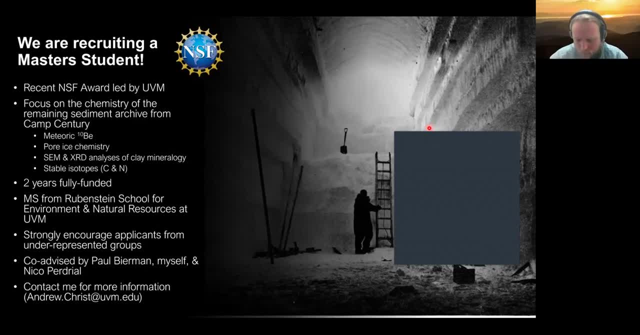 The basal borehole temperature at Camp Century. when they drilled it was far below the pressure melting point. It was around negative 10 degrees C. So I think that it's more or less local to northwestern Greenland. So there's another question that also showed up in the chat. 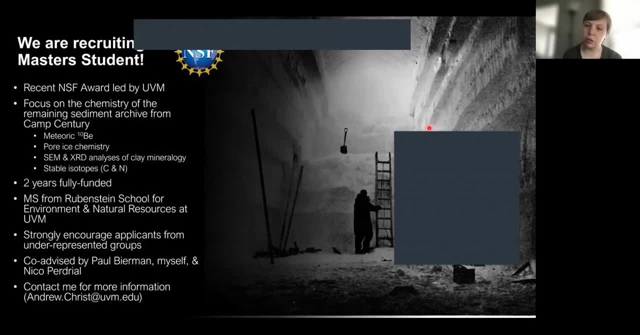 Have you used any mutual climate range methods to look at what the flora tells you about climate? We have not. We have not done that yet, And the ecosystem aspect of this project is still a work in progress. Because, number one, it was a shock. 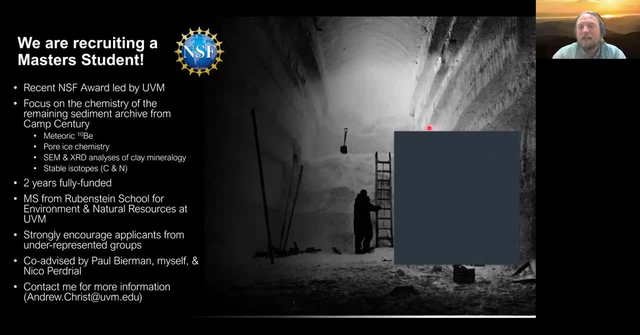 We weren't expecting to find this, And you know. so we haven't been able to look at all of the sediment yet, So we haven't been able to get a full characterization of it. And then, one more aspect of this project that is still in progress is some ancient DNA analyses. 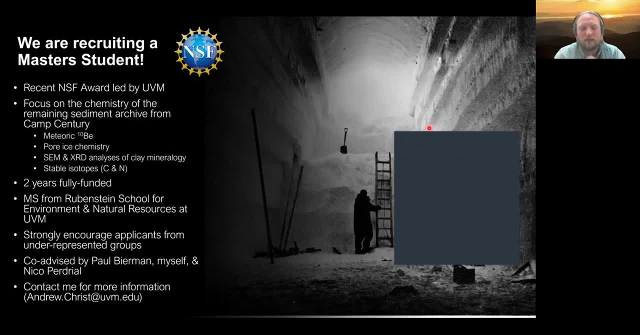 of the sediment, which would give us a better holistic view of what's in it, And then we could start thinking about how to model it and bring it into climate models. Yeah, Should be fun. We have another question that I'll add in that says such an interesting history and 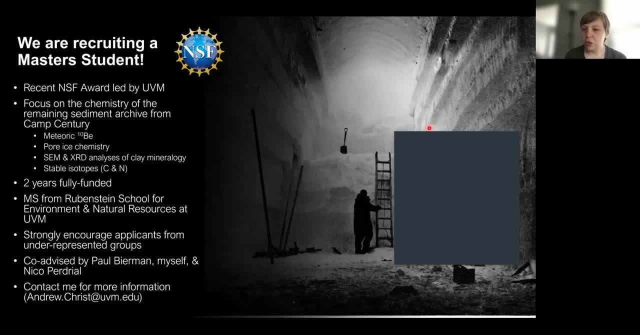 a great talk. You mentioned that there were biomolecules in the ice core basal material. Was this just DNA or has there been any work done on lipids such as plant wax? Pretty cool to find DNA though. Yeah, So just this sediment? we have just done lipid biomarkers so far. 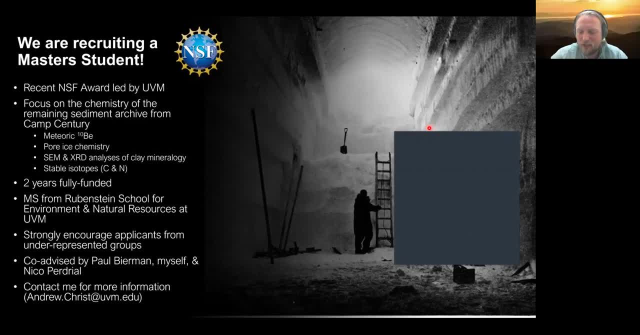 And I didn't dive too much into it. But the you know, the concentrations of those lipids and the two different units are pretty different. And again that upper diameter, then there's a lot more of it And it looks like they're better preserved than the lower, older sediment. 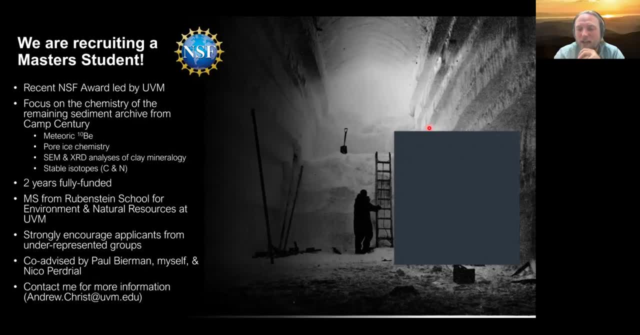 So the DNA we have, So the DNA we actually- you know it's in progress right now, But we have done the plant wax lipids. So there's another question that maybe you sort of answered with your master's student recruiting, But what do you see as the next steps for this work? 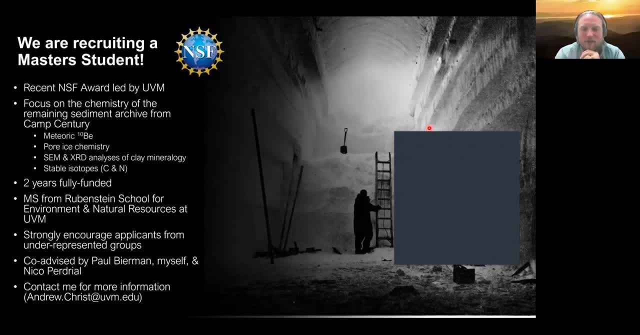 Yeah, So I just got approval from UVM over the weekend to go to Copenhagen And in very few short weeks I'm going over there to help cut samples of the remaining archives to bring them back to UVM and begin processing them and distributing them to all. 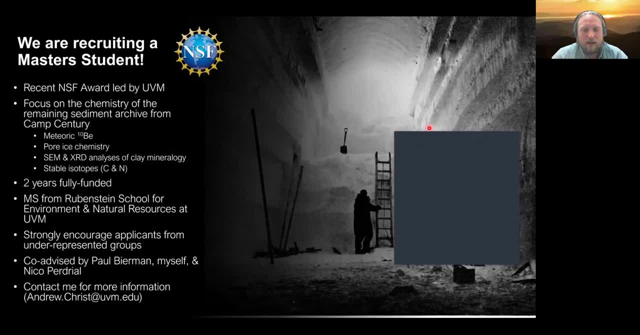 of our collaborators And that project is going to give us a much more like overarching view of what's in these sediments And it's going to allow us to get a better idea about cryostratigraphy that tells us about, you know, if there was like the permafrost conditions that may have been preserved in. 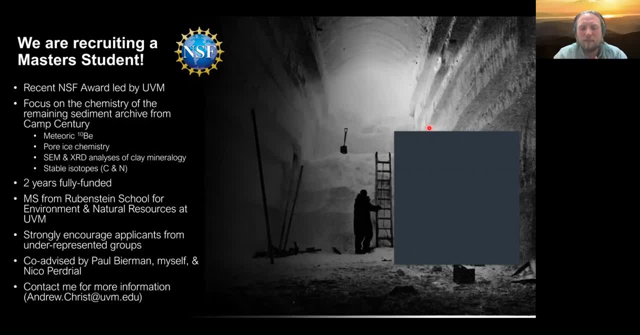 the sediment. We're also going to be able to get a better understanding of how the sediment was mixed or transported by doing additional measurements on beryllium-10 and luminescence dating And what's really. you know, what's really cool about this project is that we've been 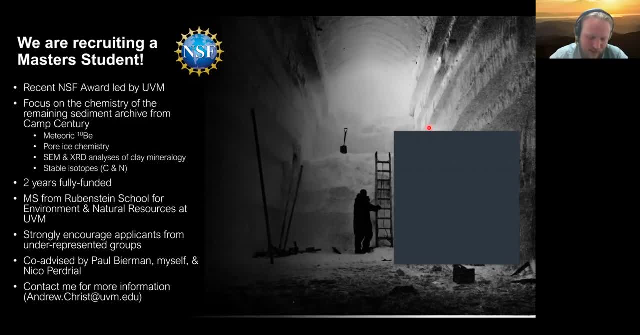 able to get pretty good results. And the other thing that I found really cool about diamicton and glacial tills is that they have minerals in them, and at such large masses that you can do analyses that can be sometimes very difficult to do. 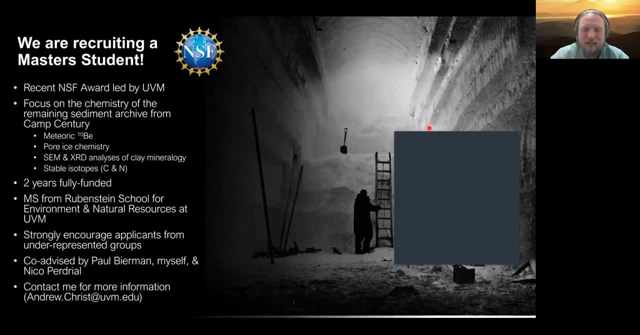 So with cosmogenic nuclide dating you need a minimum of 20 grams of clean, pure quartz to make really high precision analyses, And oftentimes that can be really challenging to get out of the sediment um sediments that are from the marine realm or river sediments that don't have a lot of quartz. 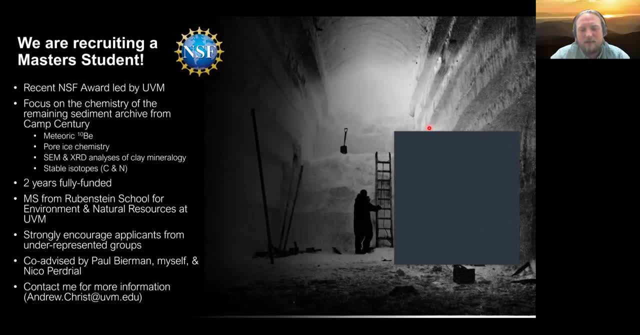 in them but diamictin. it's like we just we were able to get enough material um to do really great uh analytical work on them. so i'm excited to see see where this goes and and also to bring in a master's student who will get to hit the ground running.